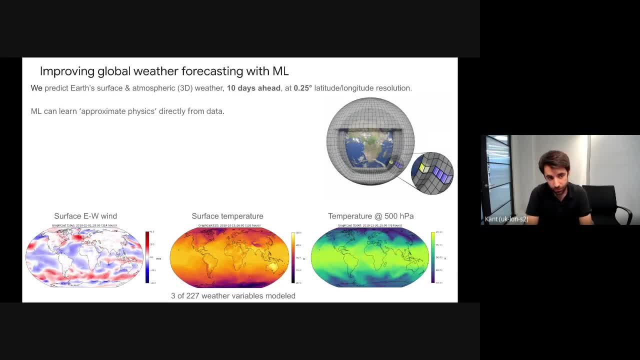 The intuition and motivation of this work is that traditionally, weather models have been essentially using classic physics, So we roughly know the exact laws of physics for the weather. If we had perfect information. of course, we don't have perfect information, both because we have imperfect sensors as well as because we have a finite compute. 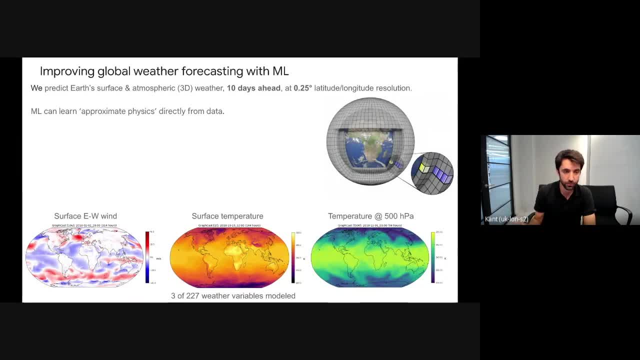 So weather researchers have had to make lots of approximations on top of this. So our hope is that machine learning can directly learn a better approximation of the weather given these constraints, because we have lots of data. In particular, we found that indeed we are able to learn more accurate, as well as much faster models than state-of-the-art NWP's numerical weather prediction models. 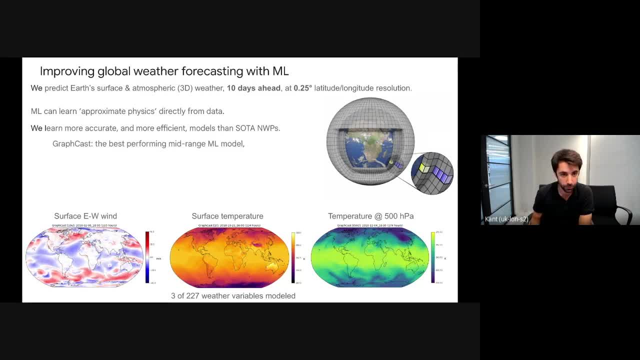 And we present GRAFCAS, which is the best model in mid-range weather prediction, And we also present a careful comparison against the state-of-the-art NWP model, a choice from the European Weather Agency. This is particularly tricky to do given some of the circumstances. 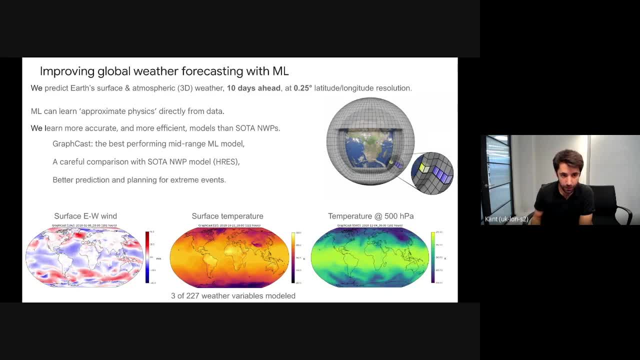 And finally, one thing that is not obvious directly is that we obtain better RMSC metrics, like usually we do in machine learning, but we also want to get better consequences for the end-user, So we also check that these better predictions in terms of metrics also translate to better prediction for extreme events. 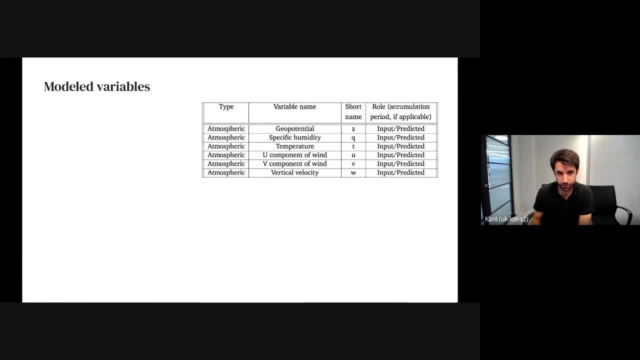 So, more concretely, the model variables, As I was saying, are different atmospheric variables, so geopotential, specific humidity, temperature and then wind in the three cardinal directions. And we model this at 37 levels of altitude and in bold you can see the ones that ECMWF, the European Weather Agency, reports in their scores. 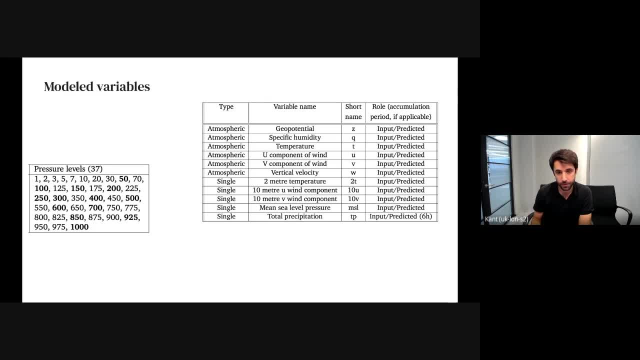 We also have surface variables which are particularly important for humans, like temperature, again wind, the pressure and also precipitation, And finally, we also have some inputs that can be directly predicted by hard-coded models, essentially like the time of day, latitude, longitude, time of the year, whether there is land or sea at a specific location and the altitude. 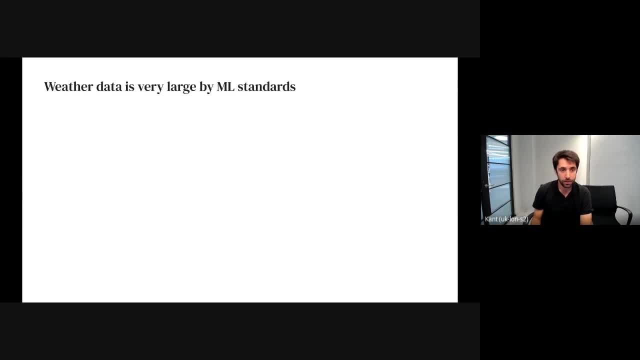 And also how much sun is radiating there. So one thing that is not obvious is that the weather is very, very large for typical machine learning standards. So here you have an image of MNIST, and here you have ImageNet, the classic computer vision benchmark. 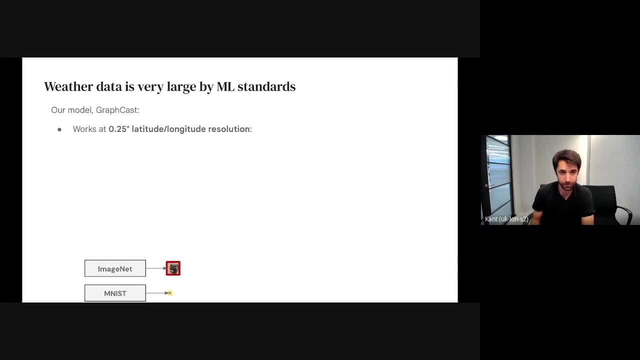 And our model, GraphCast, because it models at 0.25 degree latitude longitude resolution. it really you should think about each variable as being a very high resolution image. Not only that, but images typically have three channels: RGB. 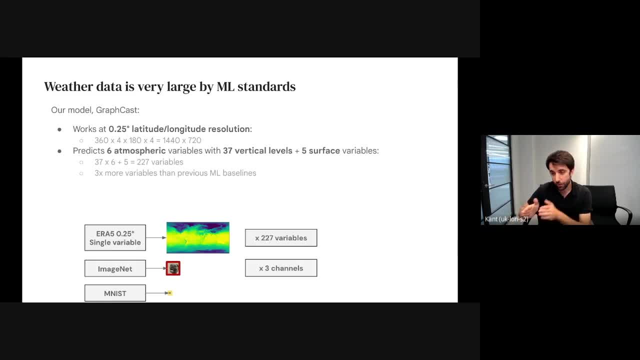 In our case, we have more than 200 variables. so now each prediction, each time step prediction, is going to be much more than a single image. And finally, because we predict 10 days ahead at six hours resolution, we actually predict kind of 40 frames, but each frame has 200 variables. 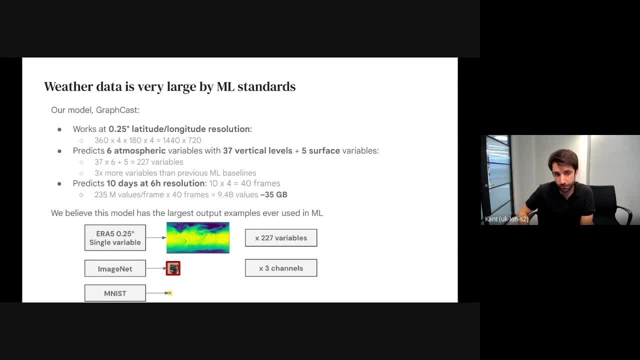 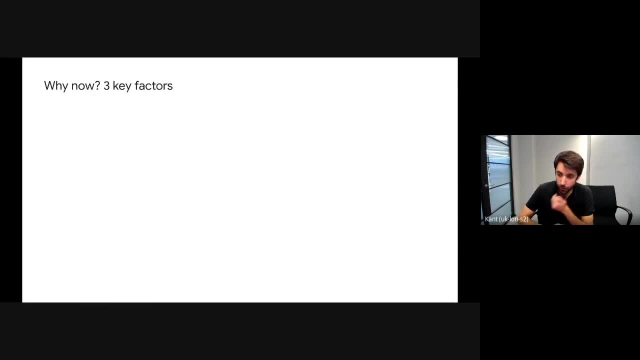 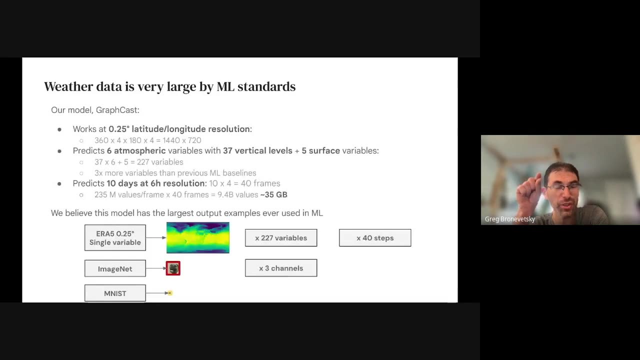 So that comes to about 35 gigs, which we believe is probably one of the largest output examples in machine learning. So my question is, why now? Why has this A question about the data set? So we don't have weather stations stationed that finely in space? 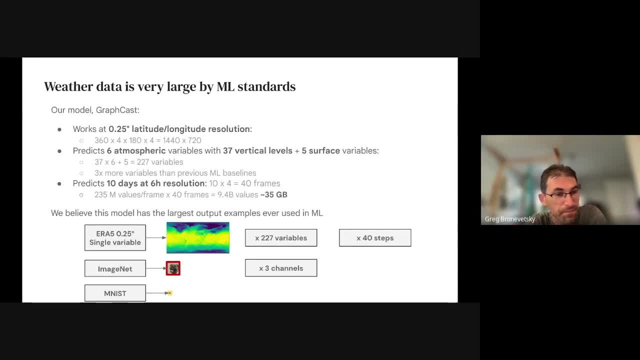 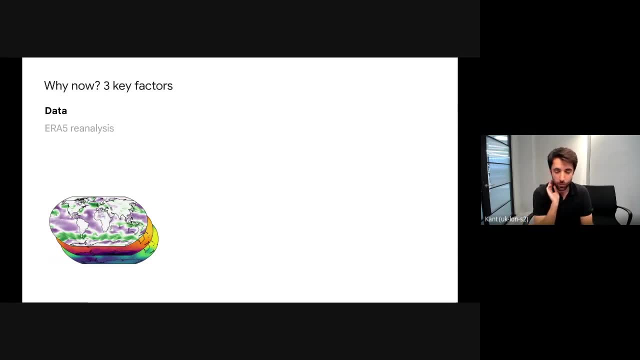 So are these, Are these re-analyses of fast weather? Yeah, yeah, exactly. This is literally the next bullet. if you're asking about the data set, Yeah, so why? now? There's three key factors, and the first one is data. 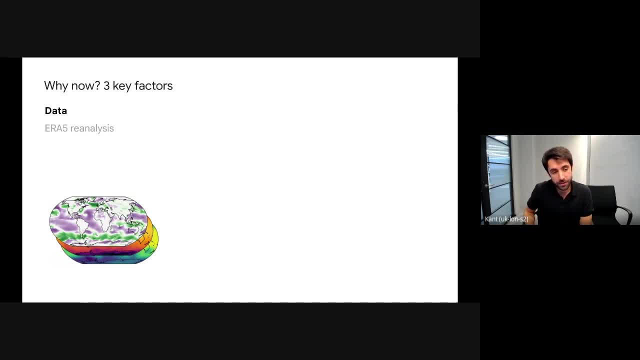 So we have available the ERA5 re-analysis, which is provided by the European Weather Agency, And it's worth noting that this is a simulation. so a simulation basically means going from raw weather sensors- right like satellites, like globes, things like this, or like ground measurements, to the kind of an estimation of the true weather state. 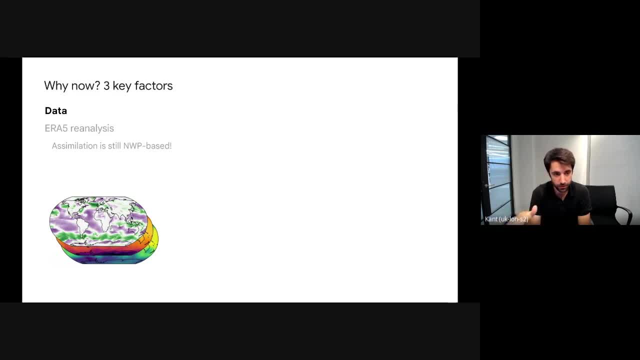 This is still based on classic physics and this is not based on machine learning. So we take kind of an estimation of this and re-analyze more than 40 years back. So we have a massive data set in terms of size, And that's why that's one of the key factors in deep learning typically. 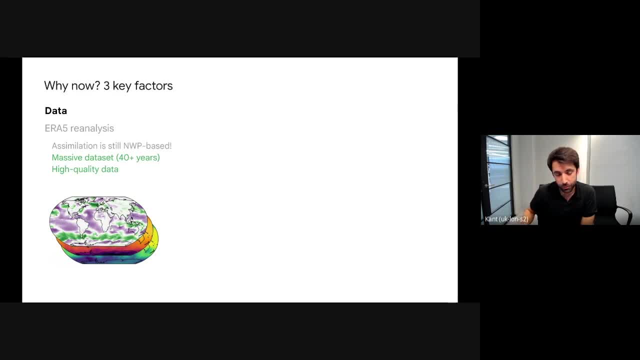 And it's also very high quality data because there's been a lot of compute effort gone into or amortized into this data set. The second key factor is compute. As you know, it's now more and more useful for getting performance and, in particular, we train on 32 TPUs. 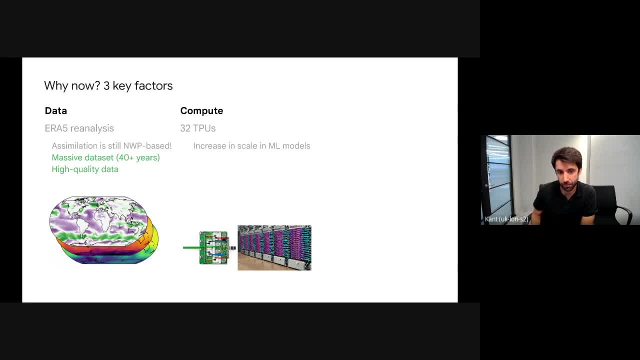 And this just goes along the line of increasing scale in machine learning models. Our model itself is quite small but, as I was saying, each input-output example is very, very big. so we really need the compute. But note that this compute is different than the typical compute in weather models. 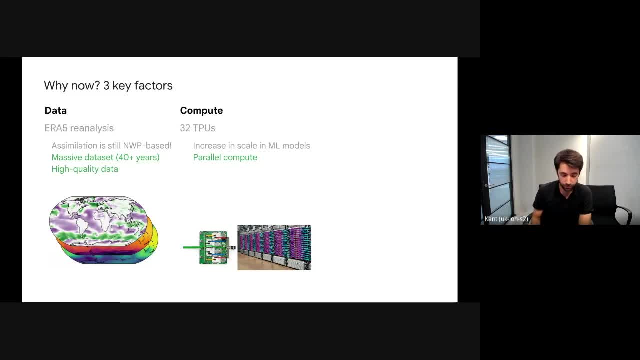 So before weather models we're using servers of around 10,000 CPUs And now we just use a few TPUs. in order to train And at inference time we only need a single TPU, which for non-Googlers is essentially like a high-end GPU. 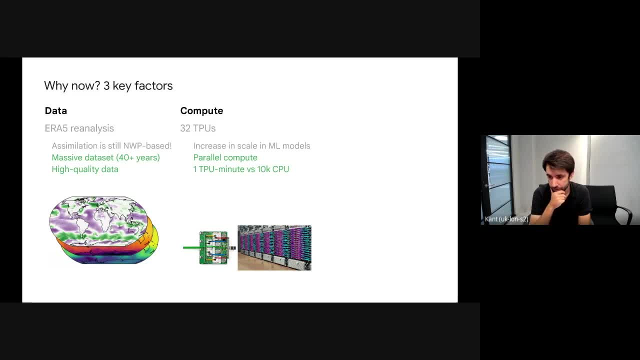 And we can do in one minute what it used to take. We can run a server around one hour on thousands of CPUs, And this is because, again, we leverage parallel compute. And the third thing is progress in deep learning algorithms. In particular, we built on graph neural networks. 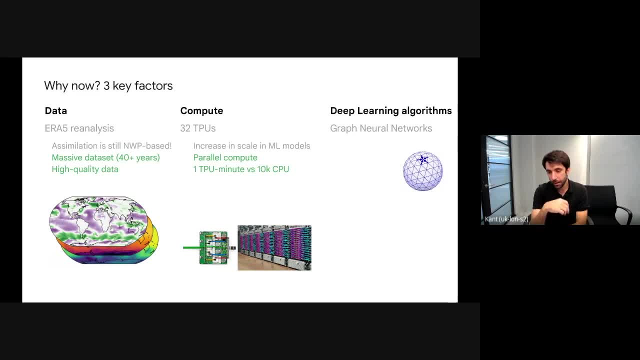 So essentially, we are going to build a mesh around the Earth and think about this as a graph And essentially, the weather is going to inform nearby weather states by passing messages And essentially, the weather is going to inform nearby weather states by passing messages. 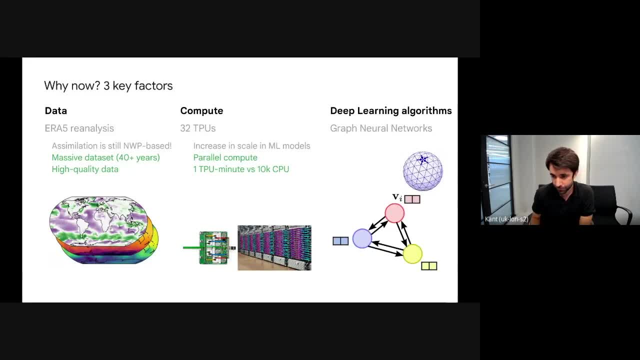 along this graph. So the kind of short story of how graph neural networks work is: they have a latent vector on each node in the graph and they also have a latent vector on each edge in the graph, and nodes inform their neighbors and so they update their own latent vectors by sending. 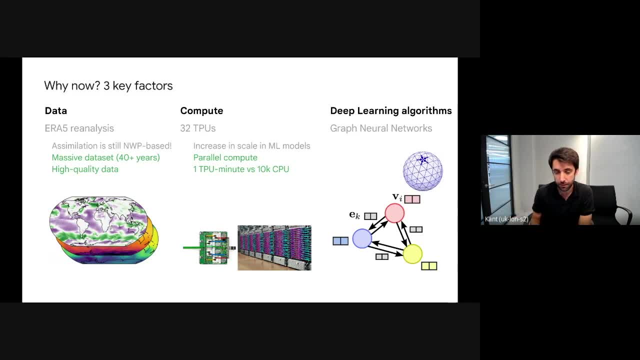 messages to nearby neighbors and then updating themselves based on their received vectors. So why do we build on graph neural networks? They have, in particular, key inductive biases that we'd like from weather. One inductive bias, for instance, is locality, because nodes only 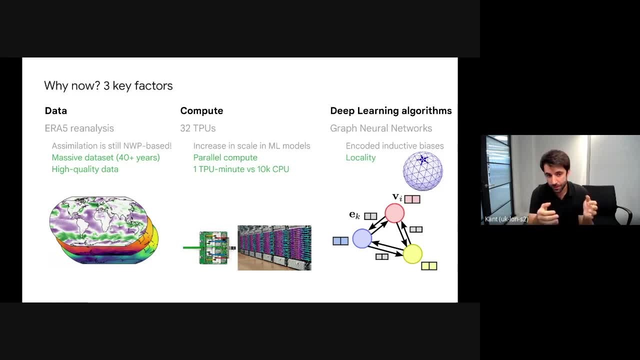 send messages to their neighbors. We are essentially encoding the fact that weather is local, and so in a short period, the weather in London is only mostly going to depend on the weather in the UK. It's not going to depend on the weather in Brazil in a short period of time. 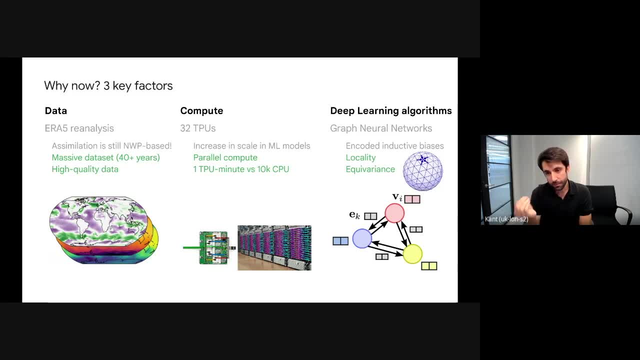 And the second thing is equivariance. So that means that because we reused the same parameters, the same neural networks on all the nodes in the graph, we're essentially encoding that the weather function is the same in the UK than it is in Brazil, than it is in Africa, And that allows us. 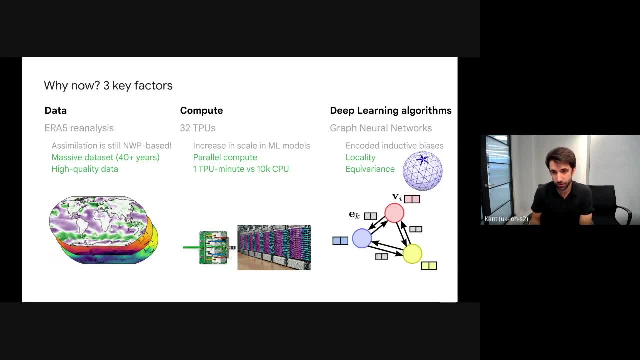 to be much more parameter efficient than if we didn't encode this inductive bias. Of course, these three key factors have been playing on the entire community, not just us. So, oops, sorry. So there's been progress in weather using CNNs also graph neural networks. 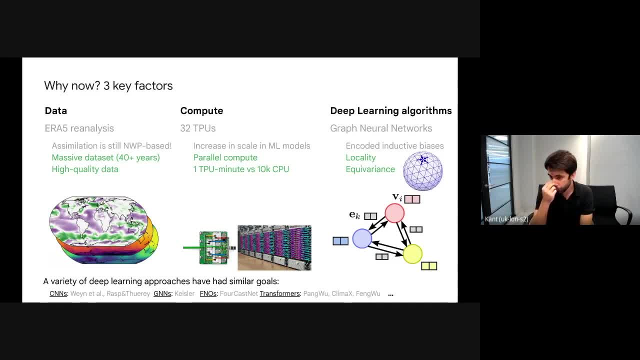 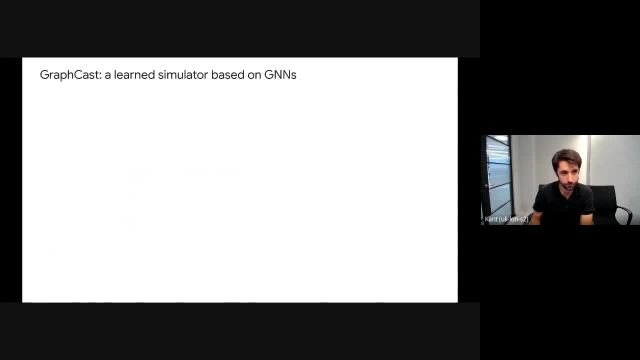 Fourier neural operators, as well as transformers, And it's really been a wave in weather prediction, using deep learning to improve upon classic physics. So let's go into more detail on how our graphcast, our model, works. In particular, we receive an input: 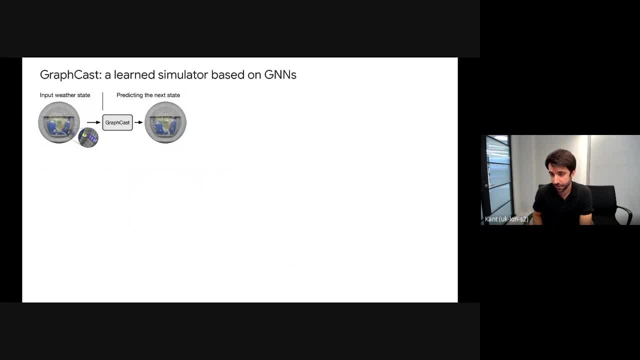 weather state and we are going to predict the next state, in particular, six hours from now. So by using graphcast, which here is shown as a black box, but it consists of three parts. So the first one, the encoder, is essentially going from the grid which, as I was saying, 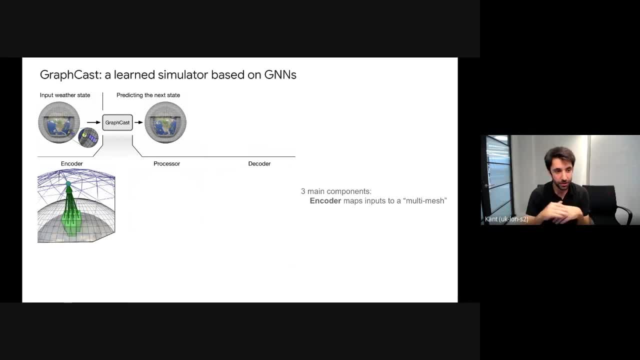 you should think about it as kind of an image, so a rectangular image. But this rectangular image is not uniformly distributed around the Earth, It doesn't know about kind of the spherical properties, the spherical geometry of the Earth, So we have to map it up to a mesh And so this essentially: 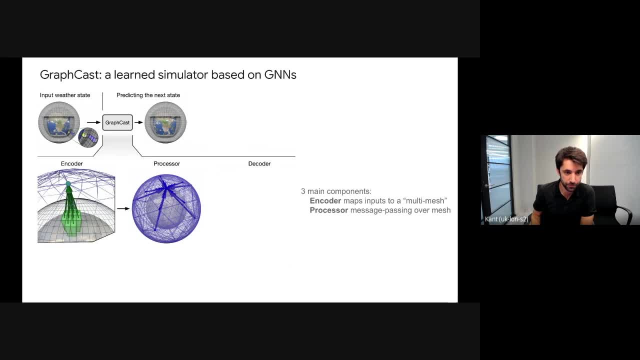 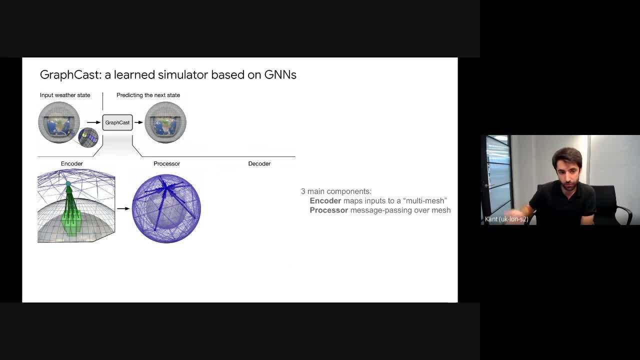 Then we use a processor which essentially propagates the information around the mesh and informs, and predicts a latent vector that informs about the next state of the weather, And finally we go back to the grid, because that's where the predictions are needed. And so we have a decoder. 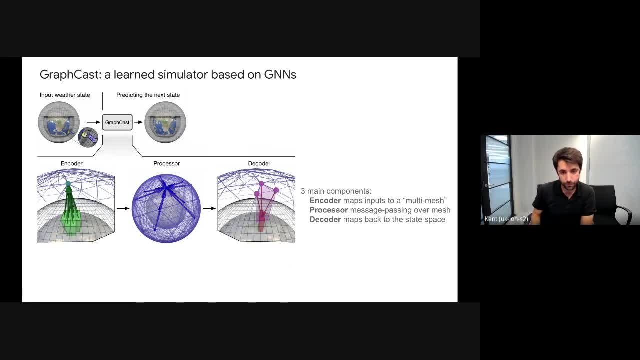 that decodes from the mesh back to the grid. This mesh that I was telling you before is actually what we call a multi-mesh. So essentially, we have a few edges that propagate the information very far and many edges that propagate the information locally. 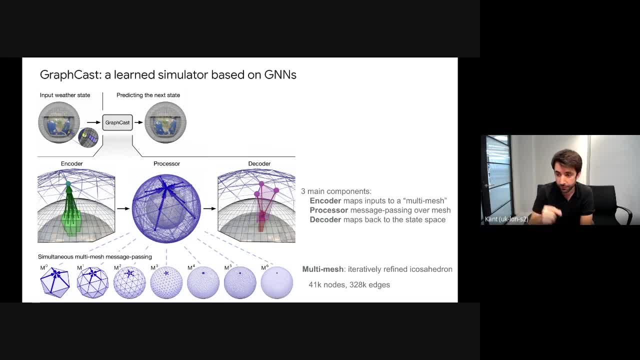 And how this is made is we take an icosahedron and we iteratively divide each triangle into four smaller triangles, And we do this up to six times, And so we're going to have kind of a few nodes that propagate the information far, and then many, many edges that propagate the information. 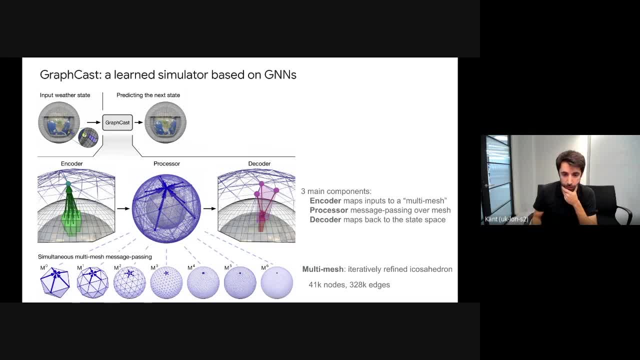 locally And we kind of pull all these type of edges together, resulting in more than 40,000 nodes and 300,000 edges, And so we have a multi-mesh, And so we have a multi-mesh, And so we have a. 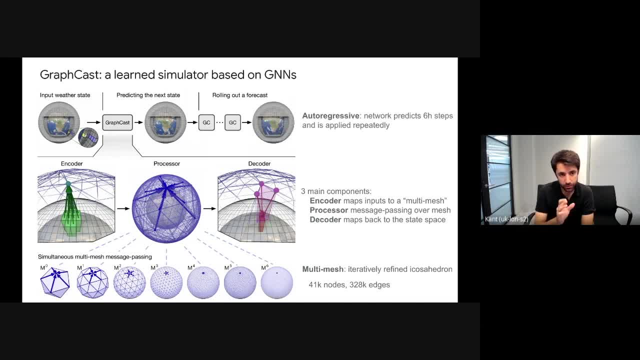 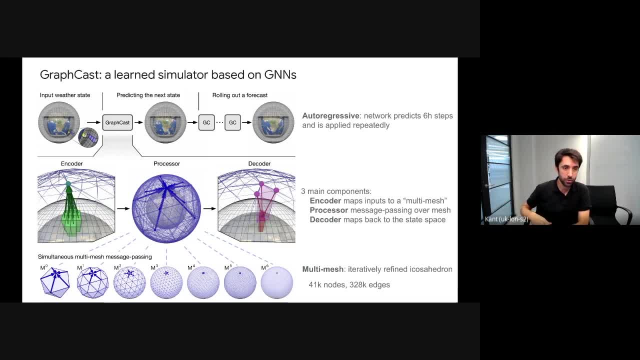 be the same as the weather function in the future. So really, if we want to predict 10 days ahead, we don't use a single neural network call that predicts directly 10 days ahead. What we do is we predict six hours at a time, 40 times, And we train for this autoregressive training. So 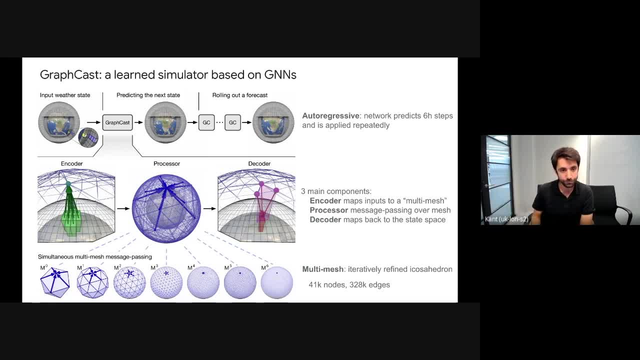 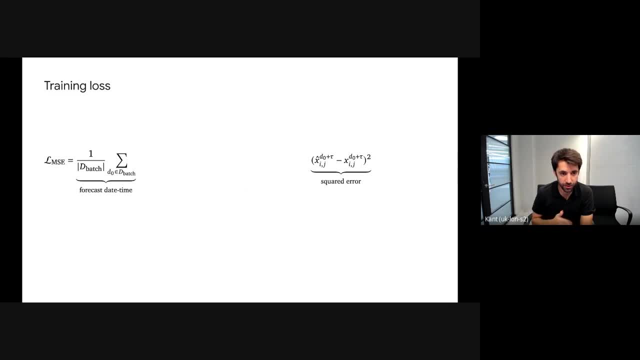 essentially applying the function multiple times to work well. Our training loss is essentially: it means: And the average essentially happens over the forecast time, So we have about 40 years of data. We also have to average over lead time, So we train the model to do well. 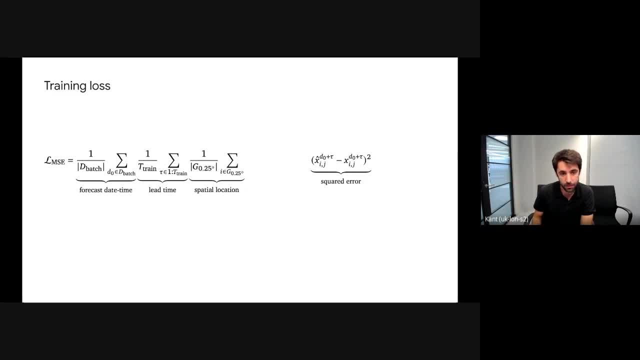 both at six hours, at 12 hours and at 18 hours, et cetera. And we also average over the entire globe And again, over variables. We have more than 200 variables, So we also have to average over them. But comparing variables is quite hard, right? You cannot just output this directly. 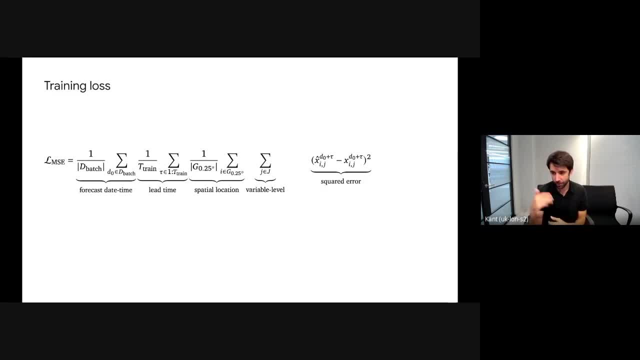 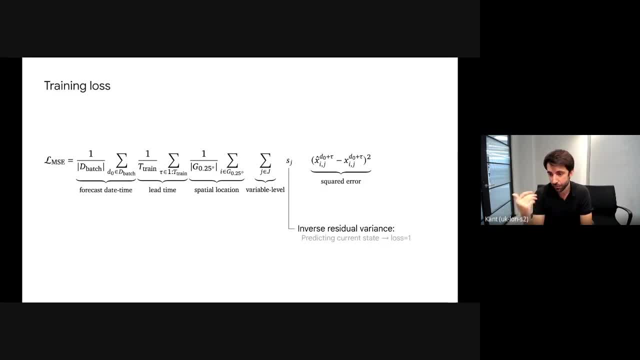 weight them, And one way we weight them is by using the inverse residual variance. So what this means is essentially that if you were to predict the input for like if you were to predict the present state for the weather six hours from now, on average you would get a loss of one for all. 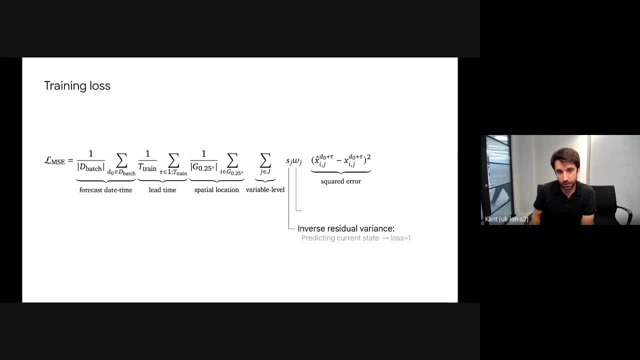 the variables in the data set, And that's what we compensate for. Then we compensate for different variable level weights. We give you a loss of one for all the variables in the data set And that's what we give them. So different levels in the atmosphere, we give them different weights. because we notice that lower levels in the atmosphere both matter more to humans and are also more impactful of the weather, because there is more higher air density there And, finally, because the grid puts more points near the poles than in the equator, you also have to compensate. 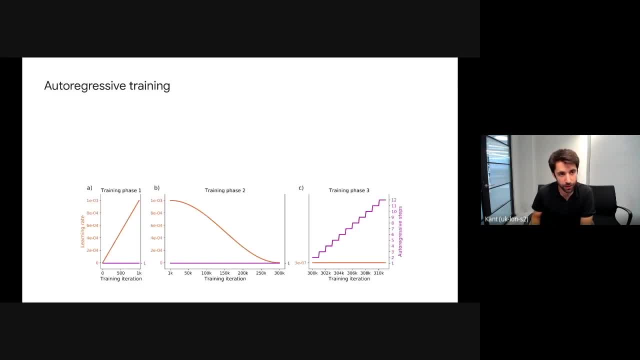 for this. As I was saying, we have autoregressive training And most of the time we spend it on training a single step. So, in particular, we do 300,000 steps at a single autoregressive step, just training the model to do well at six-hour prediction, And we do this for multiple reasons. 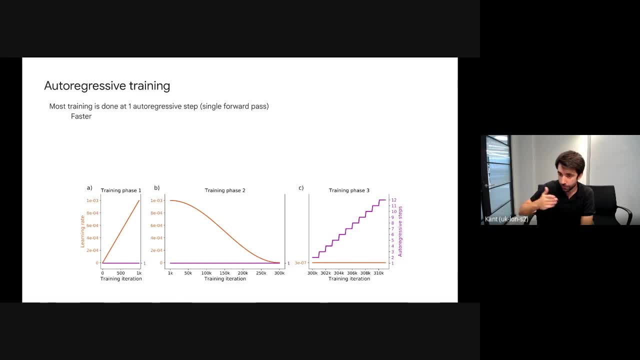 Number one is that it's faster, because if we were to train doing multiple autoregressive steps, that would mean that if we train with five autoregressive steps, it's going to take five times more, And so we found it useful to just train autoregressive with a single step. 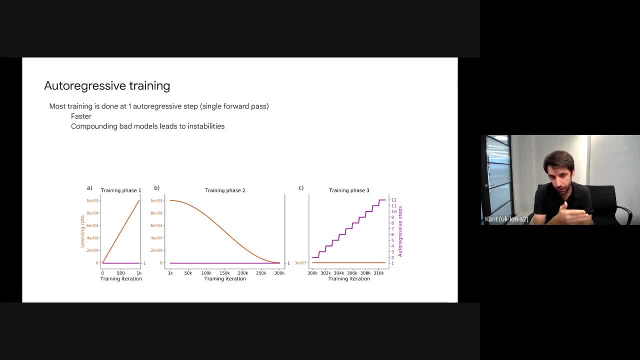 And the second one is that if you start with a very bad model and you train it with an autoregressive model from the beginning, this can lead to instabilities. So we wait until we have a very good model before starting to train autoregressively And this process takes about. 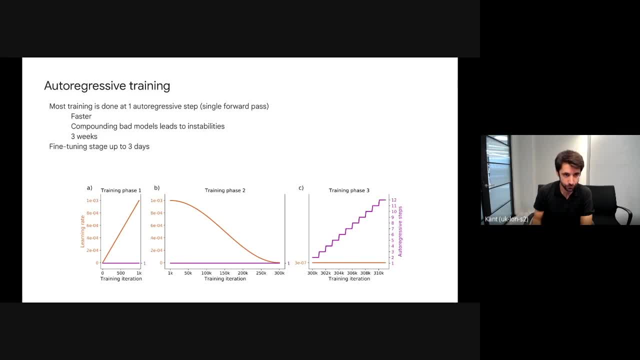 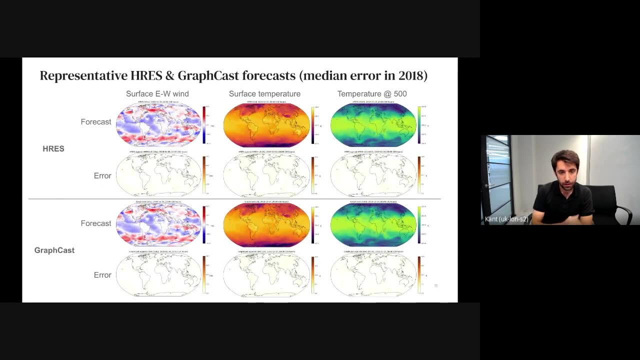 three weeks of training, so it's quite compute intensive, And then we fine-tune up to three days. So essentially we do up to 12 steps, 12 autoregressive steps, because it's six-hour prediction And this process takes up to one week. So these are the predictions coming out of 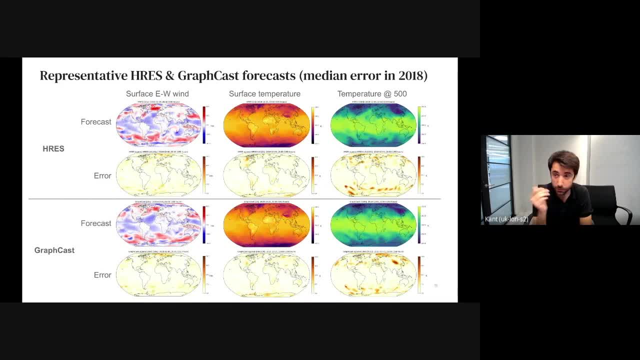 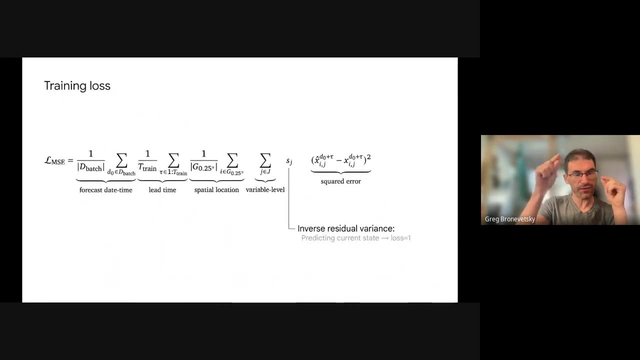 the training of our model. You can see that they look. I have a question on setting of approach. So how did you mesh it? Because you kind of quickly went through it, but it seems like it's an important part of it. One is if you can go back to the picture. it seems like it's a mesh that's different. I mean. 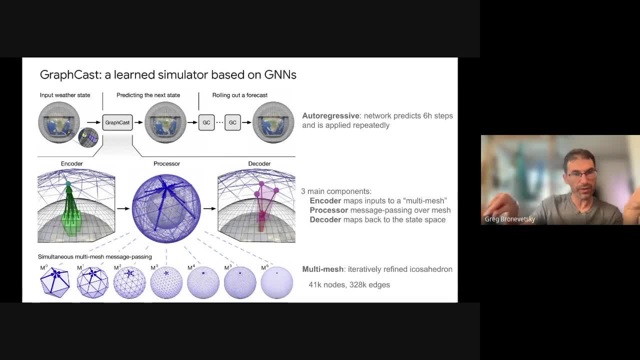 the mesh cells are smaller on poles than on the equator. So why that choice? Because wouldn't it bias your model compared to like a hex? Exactly, exactly. So that's why we have the mesh. So the grid is given to us by kind of the problem setting. So the weather community. 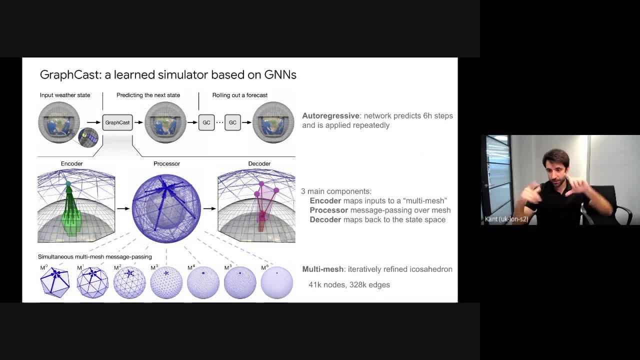 they evaluate in different ways, But the most popular way is evaluating in the grid, this rectangular image that I was showing before And that has more points nearby the poles, And the density near the poles is very high compared to the points in the equator. 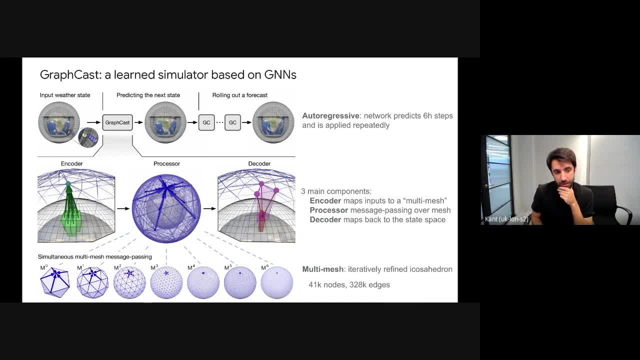 And that would bias our model. So that's why we create the mesh. And if you look at the mesh, the mesh is more uniform around the globe, right? And so the mesh doesn't have higher density in some places than others. The mesh, you can find it. 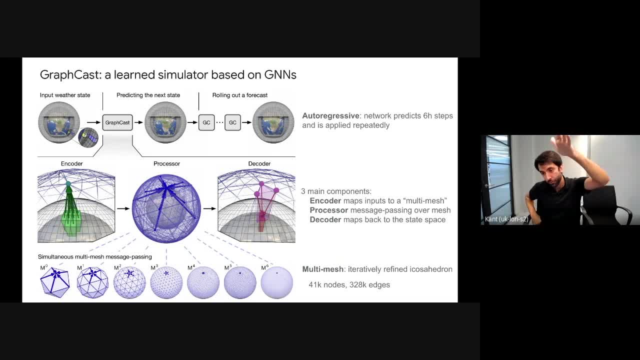 That helps a lot In the bottom row, And so we first move to this kind of more uniform distribution of nodes, We propagate the information there, and then we go back to the grid, And the grid is kind of problem-specified. We cannot change it. Okay, And that's how you're dealing with. 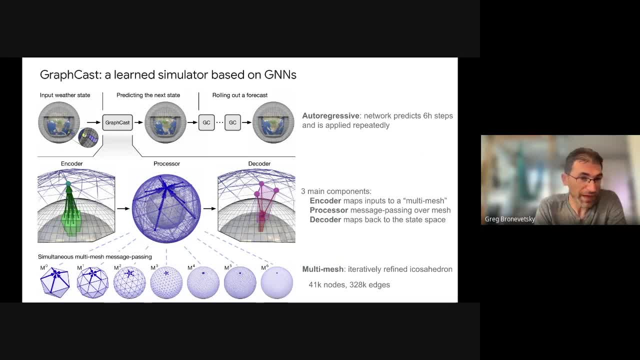 speed of causality, Because for every causal factor you're going to have different speeds, but you have a mesh for every speed. Yeah, exactly, Exactly. So we think that some processes move faster and some processes or smoother than others, And so that's why we have different layers of the mesh. 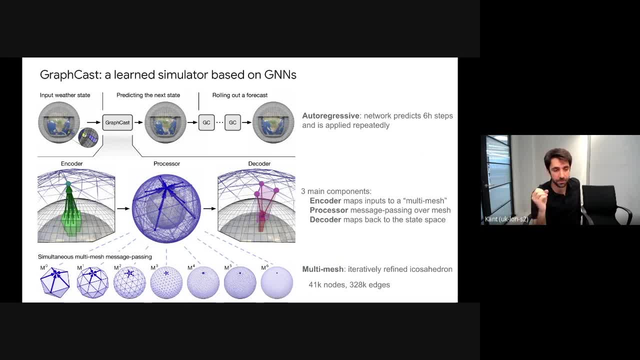 All these edges happen simultaneously, So all the message passings happen simultaneously, both the long edges and the short edges, And the model learns to use all the different edge lengths to propagate different types of information. Okay, And then one more thing: You don't have a notion explicitly here of time or history. 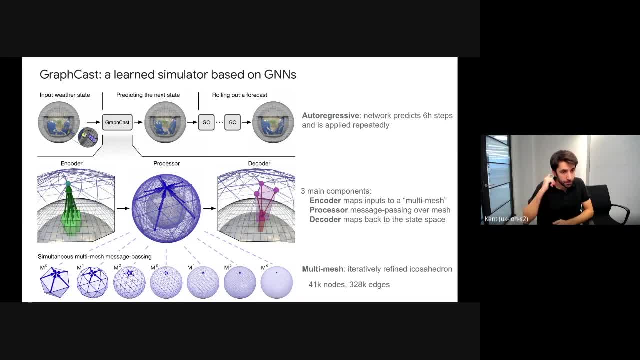 dependence is, but you have longer distances for. so it means your maximum distance of history is one. well, I guess quarter of the way around the Earth, if I get it correctly. Is that right And is that good enough? Yeah, that's a good question. So technically, 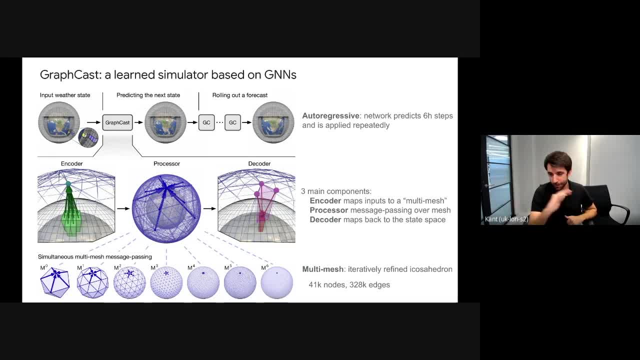 we have 16 message passing steps, So there is plenty of time to go around the globe multiple times So the model can learn some non-physical, non-physically plausible physics. It just learns about kind of data correlation and data information. It's not bottlenecked by. 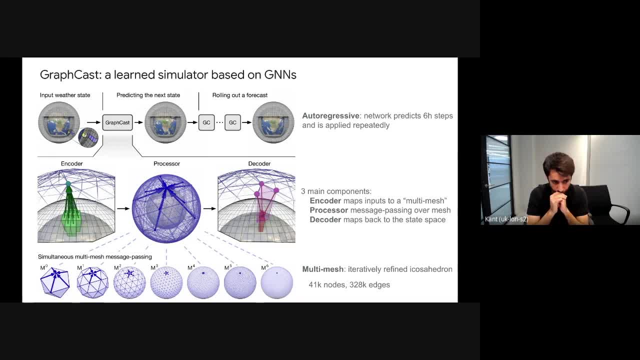 by kind of speed of sound or things like this. Now that we're on the topic of temporal things, we actually- the input of the model is actually not just the present, but the present and six hours before. In theory, weather is Markovian, but we found that probably due to partial information. 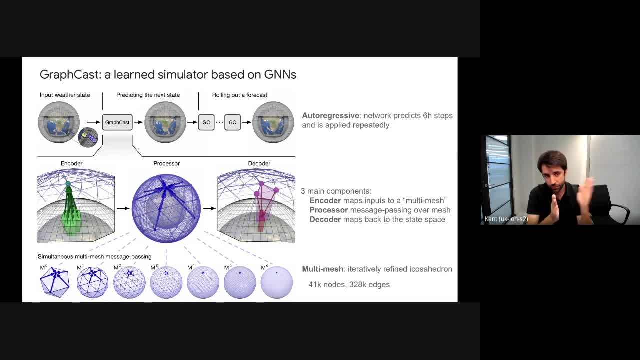 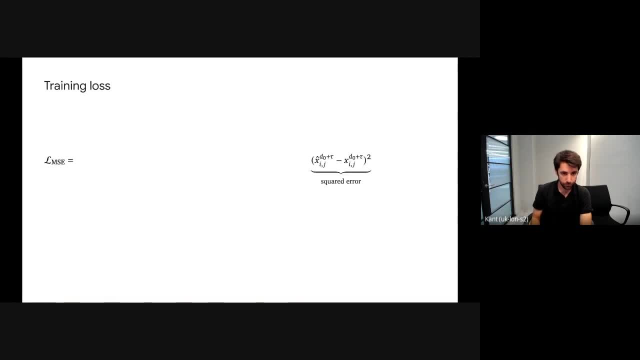 and kind of issues with data simulation. it was useful to have two time steps so that the model knows a bit about the dynamics of the model of the weather as well. Okay, Actually, maybe it's a good time to ask this. So it's the whole Earth, 40 years, but for the Earth. 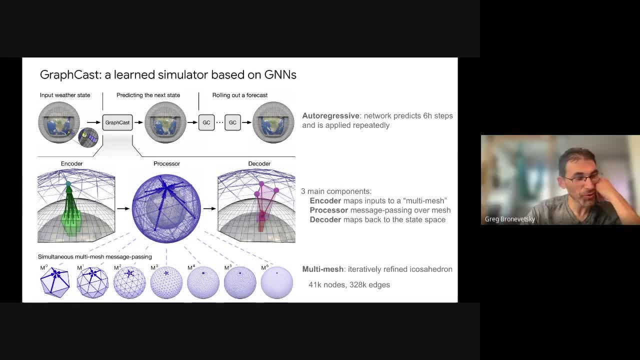 40 years is not very much. So how to what? I guess how badly is overfitting hitting you? Because it is just 40 years of a complex system. Yeah, Yeah, Yeah. So that it's interesting because four years sounds to some people may sound initially like a lot, but actually in. 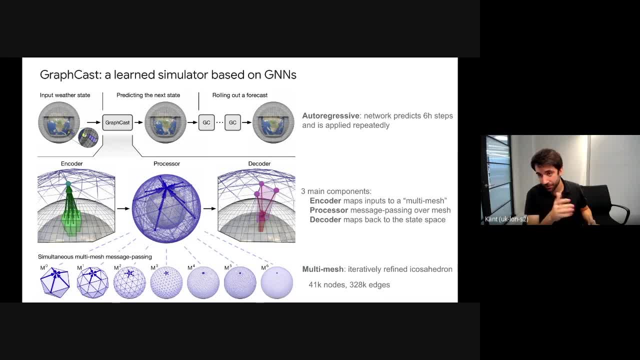 terms of time steps at six hours, there's not that many examples. But, crucially, each example is super, super rich in information. There's lots and lots of losses. So actually it's in terms of number of targets, if you think about it. per time step, it's not that many. there's not that many. 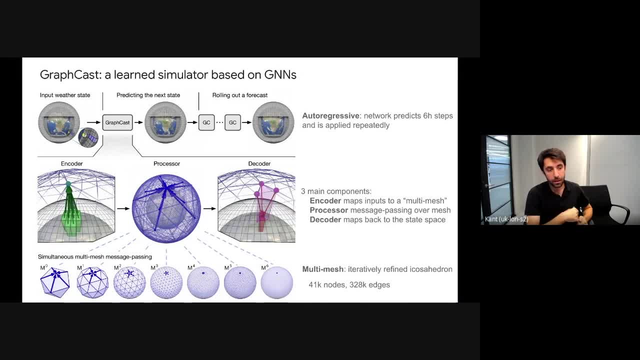 time steps. but in terms of actual targets, there is lots of targets. We found that before doing autoregressive training, so if we were directly predicting, let's say, 10 days ahead, there was huge overfitting. Once we moved to autoregressive training, the overfitting diminished a lot. We 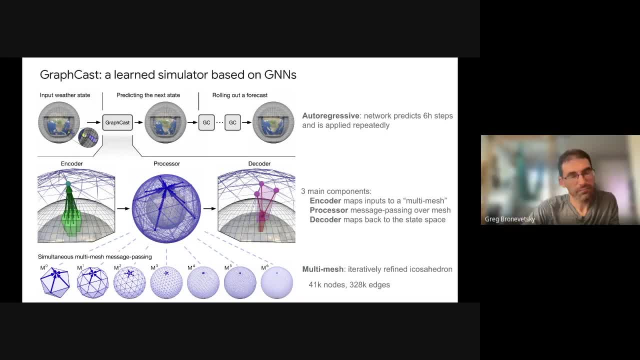 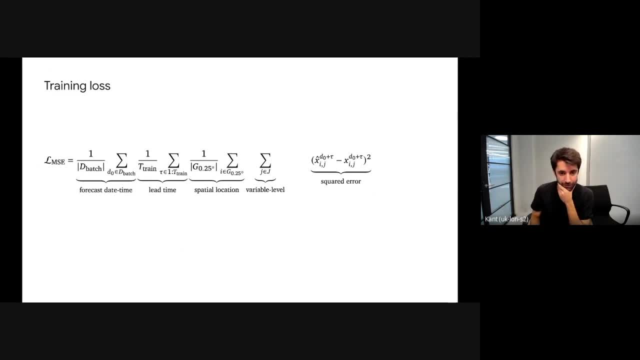 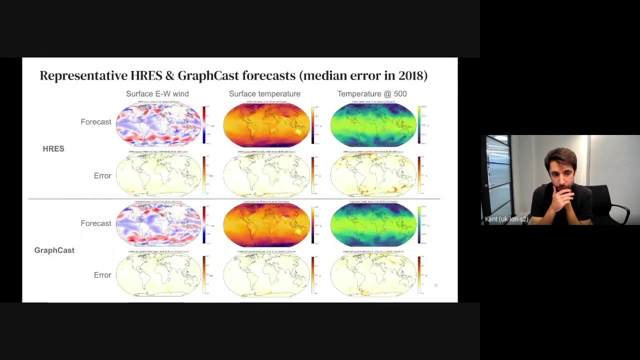 found that, in terms of the data set, it's not that much of a penalty, but we don't think we're overfitting too much. All right, Thank you. Yeah, Because the data set is actually huge in terms of number of targets, Right, Yeah, It's a good question. Okay, So, oops, Yeah, So, as I was, 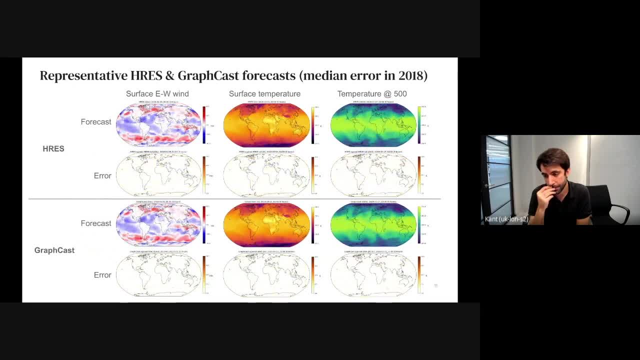 saying: we have this forecast, which again is the median error in 2018, which was our test year, And you can see that the predictions of graph cuts in the bottom look reasonable compared to the ones in the bottom, And you can see the errors also, of course, increase with time And hopefully you. 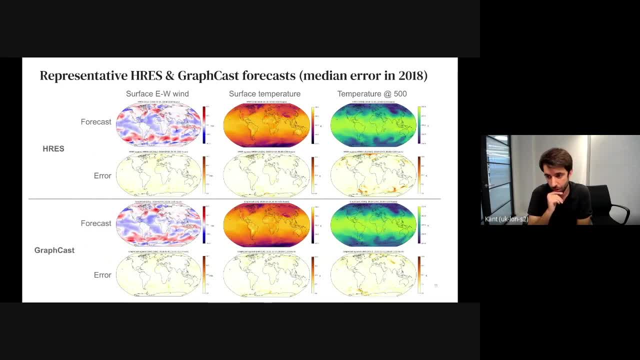 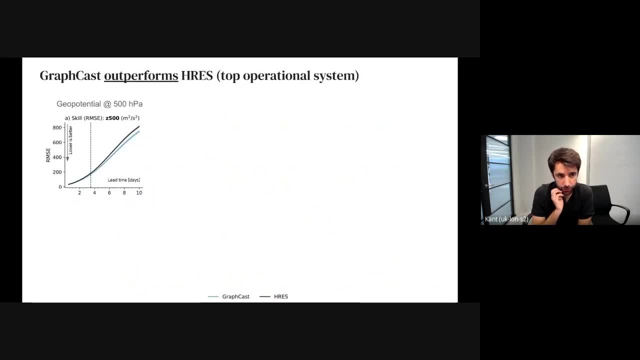 can see that the errors in age rate on the top are slightly higher than those of graph cuts. This is hard to see in images, so let's look at it quantitatively. Here we have a very standard metric in the weather community, which is geopotential 500.. 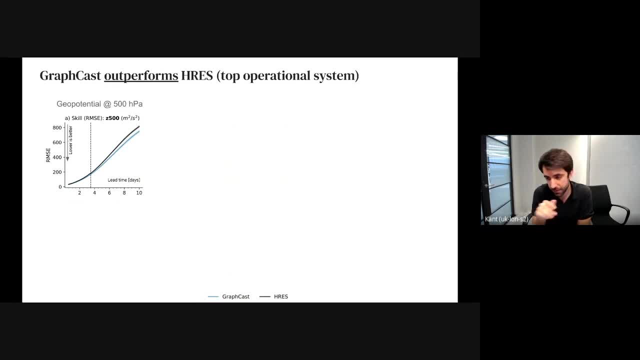 One second And then we have RMSE, so a measure of the error in terms of time And of course it's of course the average, the least。 As the lead time goes on Right, And lower is better And 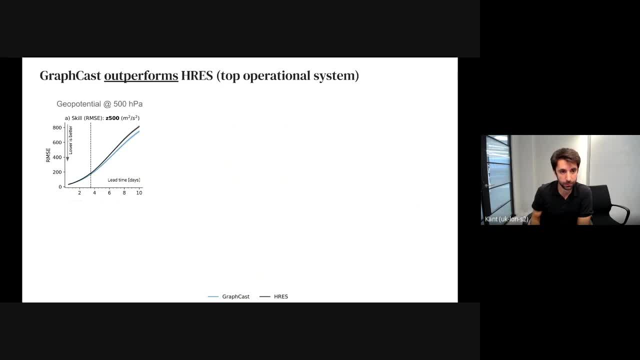 you can see that graph cuts in blue is significantly better than the interest in black. For now, this regard, the dash lines- I'm going to talk about it later- And these, of course, to kind of remove this time dependency we normalize by interest. 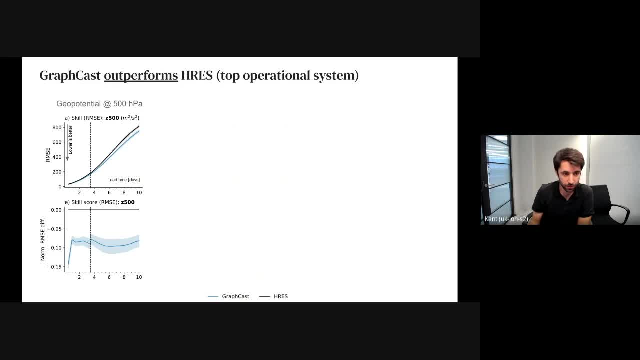 and we actually look at the percentage of improvement of graph cuts on top of interest And you can see that, for instance, for Z500 is about 10% improvement. So we have 10% improvement, lower RMSC, and this can be done for many variables like two meter temperature or surface wind or 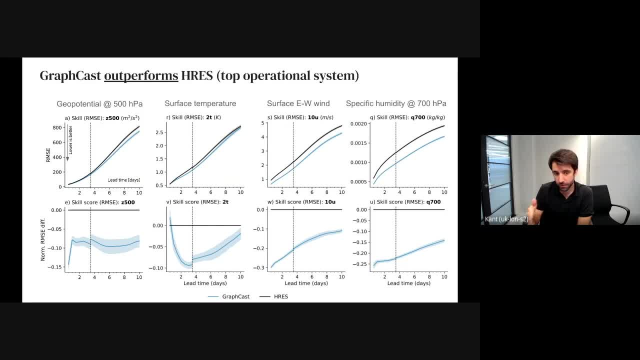 specific humidity at 700 hectopascals and for each of them we're going to have a percentage of improvement depending on the lead time. so, for instance, you can see that at 2t at the very beginning we are slightly worse and then we become about 10 percent better and then towards the end, 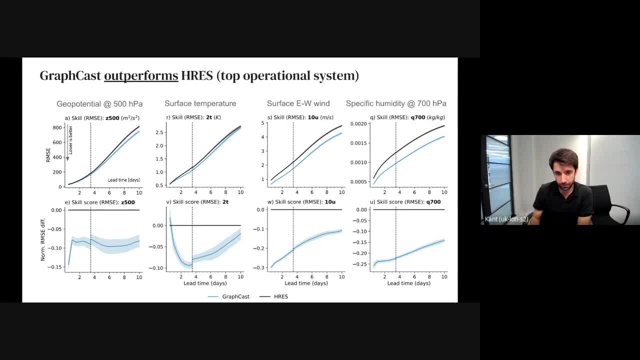 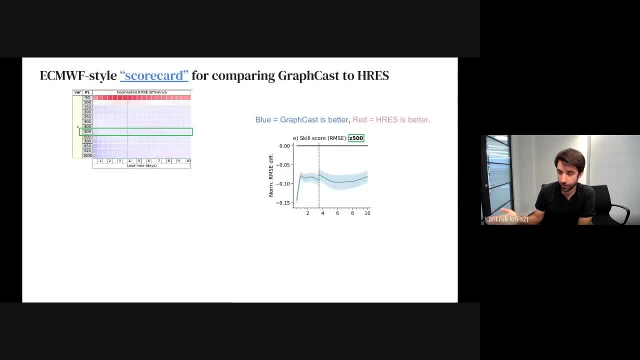 we become just slightly better, and for other variables, like the surface wind, we can be up to 30 percent better at the very beginning. but, as I was saying, there's many, many variables, so we have to find a better way of representing all this information and we take the ECMWF scorecard. 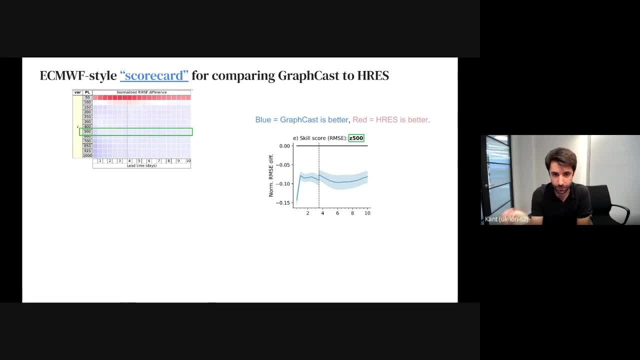 which essentially just a color map of these residual, of these relative scores. in blue you can see where graphcast is better and the deeper the blue, the better graphcast does, and the opposite, the deeper the red, the better it does. and you can see that essentially we also have lead time. 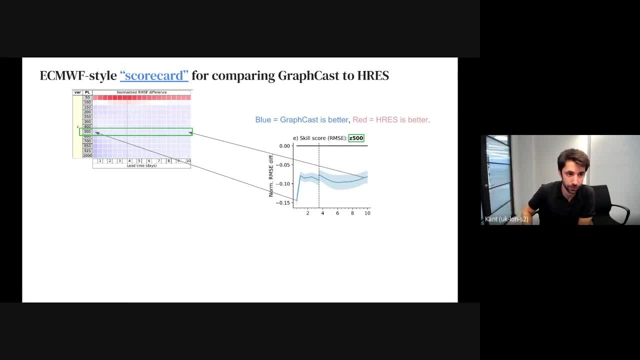 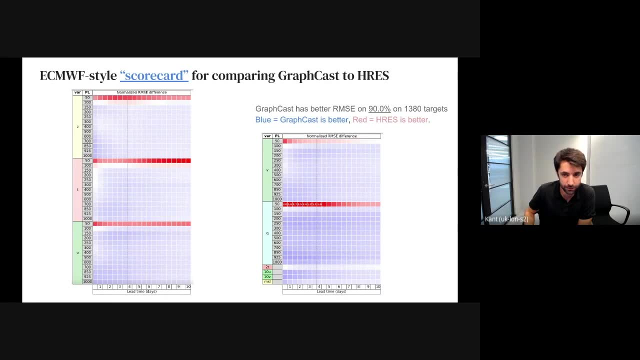 going to look towards the right and we have all the different altitude levels for geopotential, and then here we have all the different variables and lead times, leading to more than a thousand different targets, and the summary is that, essentially, graphcast does better on 90 percent. 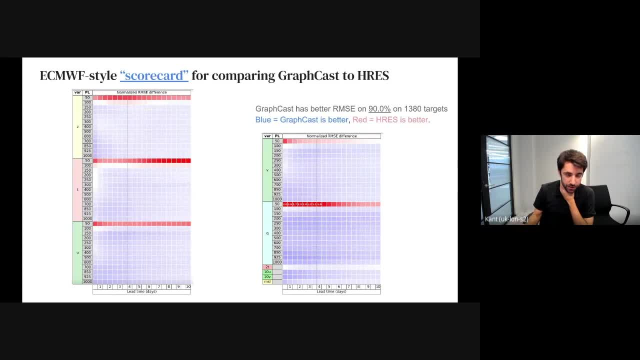 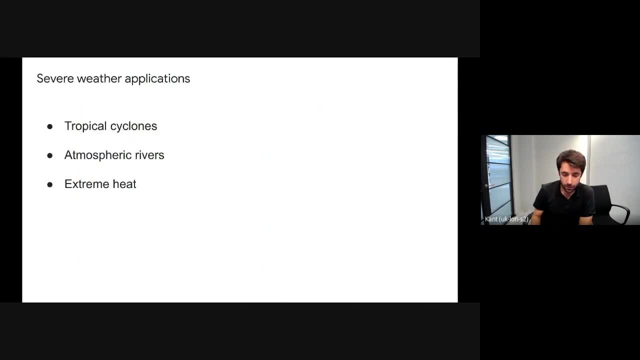 of those targets, and you can see that, especially on the lower levels, where humans care more about this well, graphcast does particularly better. so of course it's great to see that graphcast can do a great job on on these kind of RMSE metrics. however, the real world uses weather models that go far beyond these RMSE metrics, so we thought it would. 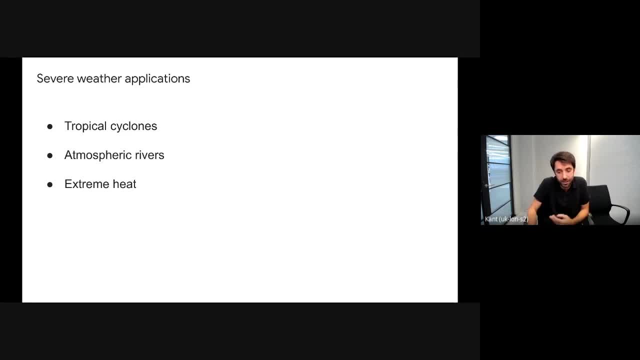 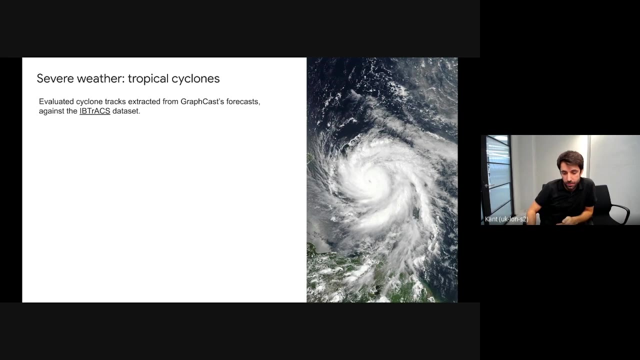 be interesting to study some of these extreme weather phenomena that heavily impacts people's lives. we decided to focus on three applications- tropical cyclones, atmospheric rivers and extreme heat- to show how graphcast performance translates to these settings. we start with tropical cyclones and we essentially re-implement. 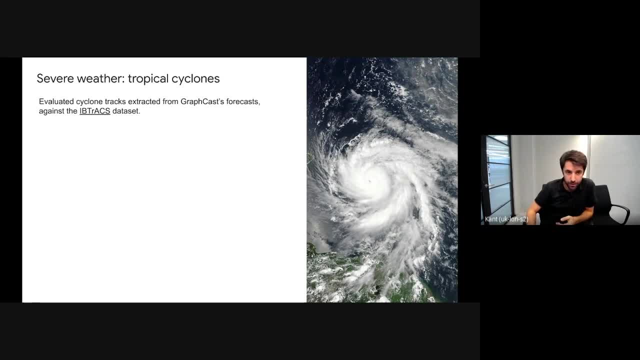 the weather agency in the european weather agency cyclone tracker and applied it to graphcast and we took the cyclones from the ivy tracks data set and in this plot you can see hurricane maria from 2017, which was one of the first terms to ever hit puerto rico and the surrounding areas. 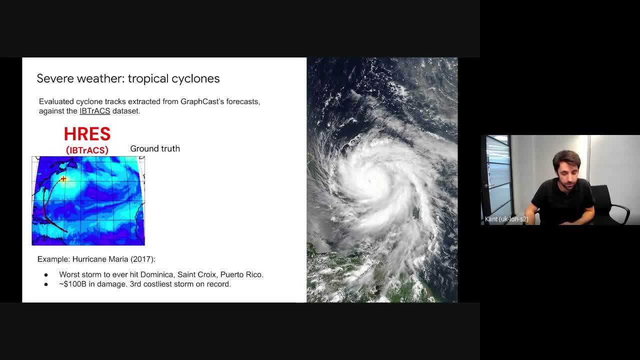 in black you can see the ground truth for five days and in red you can see the forecast for aegis. and here we observed that the aegis track totally misses the true track after a few days and the graphcast on the right is much closer to the ground truth for the full five days. 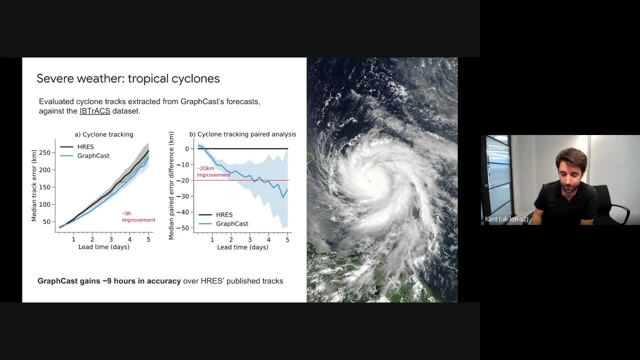 so of course it's that one was a single, a single specific date, but measuring across the years of hurricane data, yep. can i ask how do you extract cyclones? this is not really a graphcast question, but out of interest, how do you extract cyclone trajectories from your stack of 227 variables? 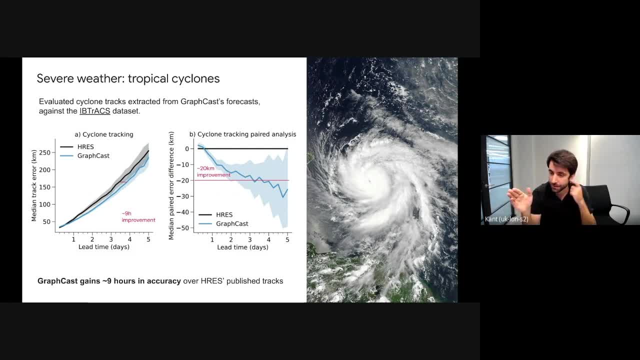 yeah, yeah. so the open, not open towards the implementation patient of the tracker. but they describe how the tracker uh looks like and so they. it's essentially a combination of mean sea level pressure and then the winds, so the center of the hurricane is essentially like a local, a local minima of. 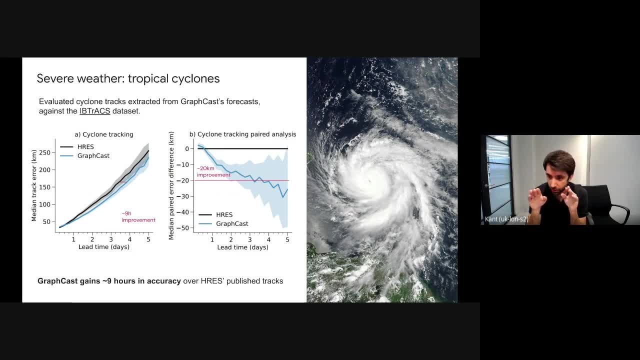 min level pressure, and there's also a few criteria on locally uh, on like, the vorticity of uh. that depends on, though, on the speed of the like, different velocities, uh nearby, and there is a uh i forgot exactly. but there's also a another criteria on the gradient, on the pressure, and so 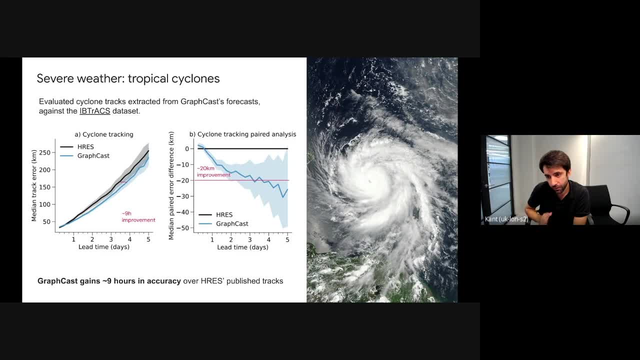 there's a few technical criteria you can follow up with you if you want on the specific, but think about it as several criteria: that the, that the local weather has to satisfy. and then you have essentially a tracker, that um, that just propagates and and and tracks the, this local minima of, of. 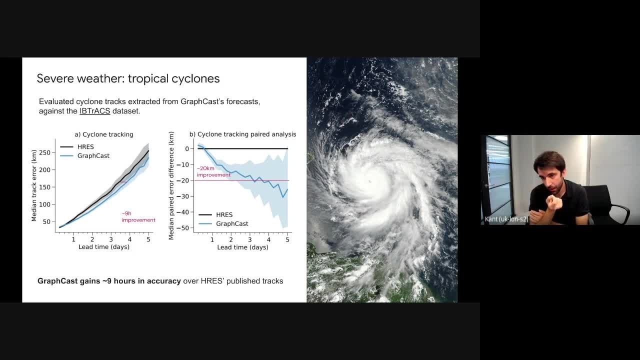 mincy level pressure to initially detect the cyclone. uh, we start from the iv tracks data set. so there's nothing in our system that predicts here there's going to be starting a cyclone. but it's very easy- well, not very easy actually, but it's. it's relatively easy to uh track the cyclone. 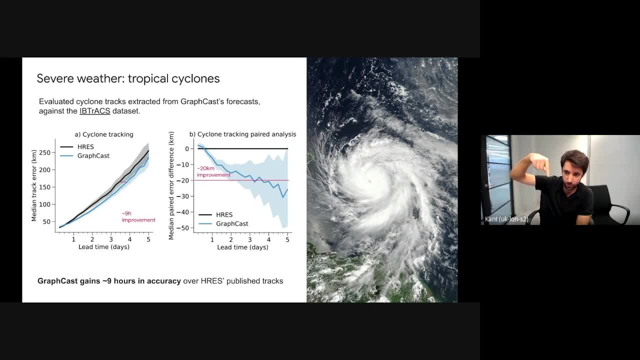 uh, once we know, okay, if we, if we're given, here is the starting a cyclone, please track it. uh, the one, the. there is enough information to know, uh, where the cyclone is. so the cyclones, it's a, it's a point in space. it's a two-dimensional cyclone. it's a two-dimensional cyclone. it's a two-dimensional. 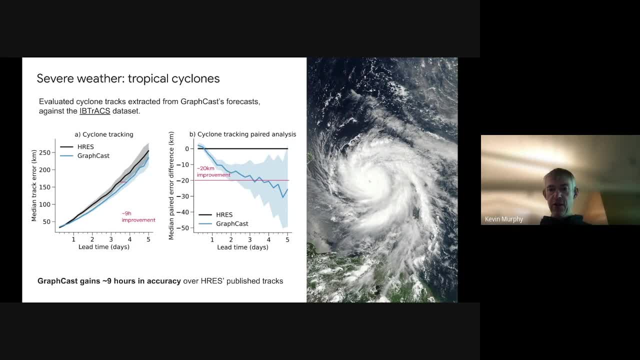 coordinate um and then the. it's a function that takes maybe the surface level variables and then spits out the, maybe the previous location, and tells you where it's going to move next. basically, yeah, exactly so, uh, you have we. so here we're talking about the center of the cyclone, yeah, but 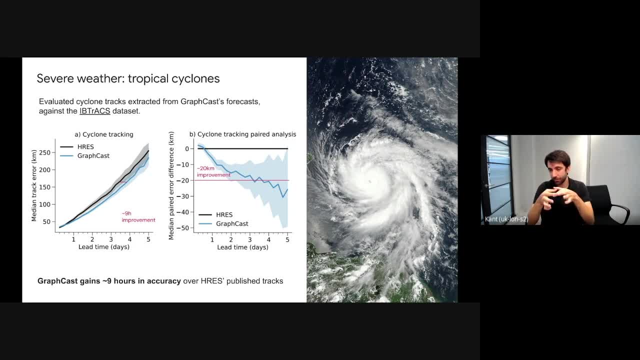 uh, to really know where the center of the cyclone is, you need to look at the nearby area, think about it, maybe like three, four degrees, and then based on the wind, for instance. uh, you know, okay, if there's a wind, if there's a cyclone, if the wind is strong, you need to know where the wind is and then the 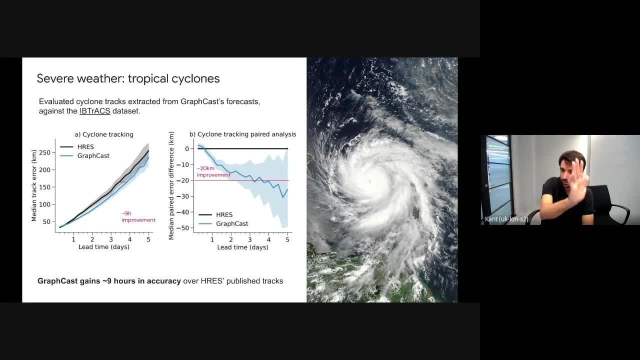 wind going east, then the cyclone had to move east. And so you estimate: oh, six hours from now the cyclone is going to be near this area. And then, near that area, you start looking for mean sea level, pressure, local minima, And then there is a very specific algorithm. 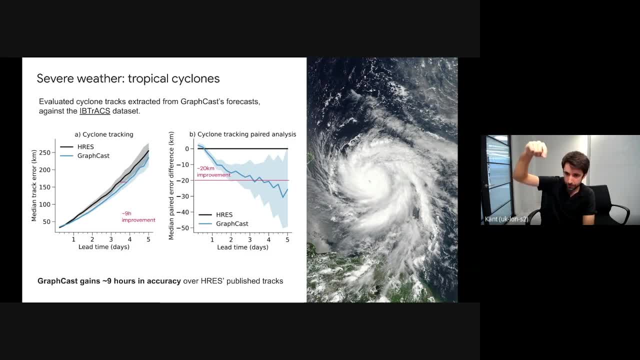 that the CNWF published, And then we essentially re-implemented that. One thing that we found is that if we literally re-implement their published tracker, it doesn't work quite as well for us, because their tracker works for their predictions, And so we had. 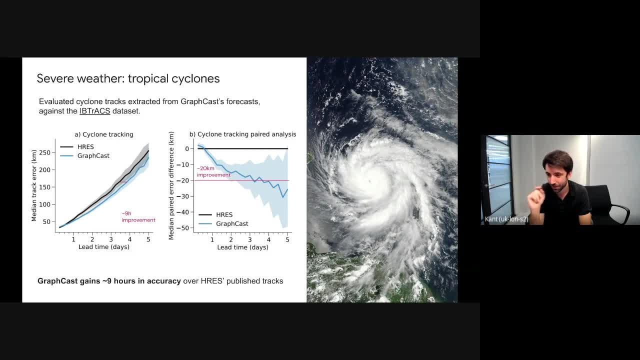 to change some of the constants. some of these magical constants like, for instance, there is different thresholds on what the cyclone has to satisfy to keep being considered a cyclone, or which points not all the local minima of mean sea level pressure are good. 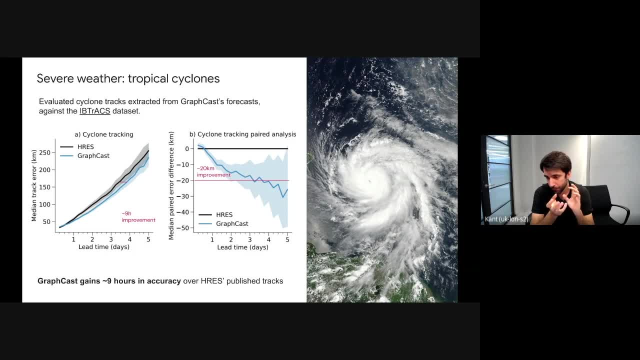 cyclone centered candidates and things like this. So we kind of search on validation data for some of these conditions for being a cyclone. Am I answering your question? There's a historical database, I guess, of previous cyclones, That's right. So the IV-TRACS data set it's literally a data set of cyclones. So 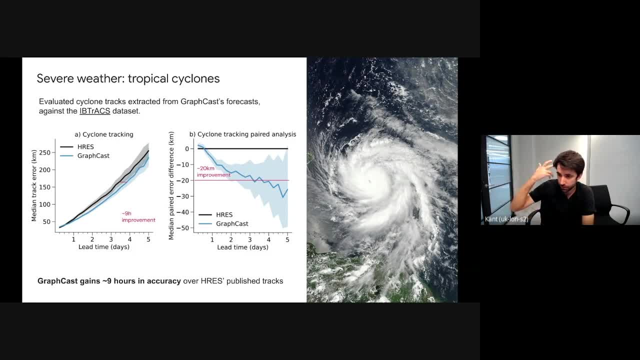 the way this is collected is they have different weather agencies around the world, And then they had all these conjectures about where the cyclone was at each time step. They don't quite agree with each other And the IV-TRACS picked a reasonable. 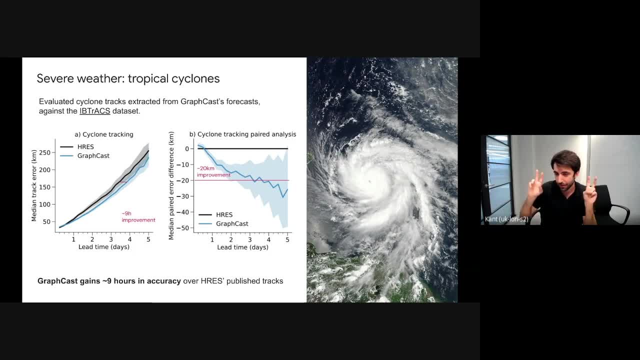 agreement between all these different weather agencies to kind of get at the gold standard on where each cyclone was at each point in time. And so we have- I forgot how many years we have, but we have probably more than 20 years- of cyclone tracks available, And that's what we use for. 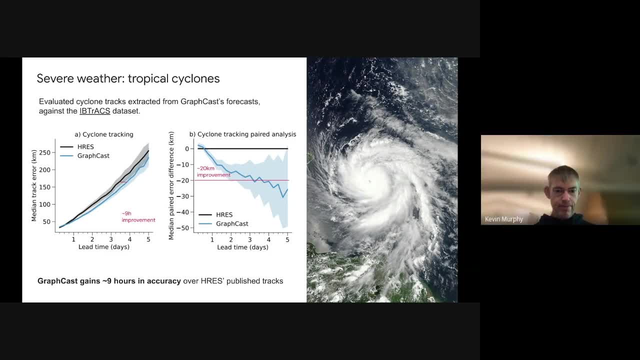 evaluating the cyclone performance. I see, Thank you, And yeah, how this looks like is it's essentially latitude, longitude, but there's also, if you're interested in cyclones in particular, there's more, a lot more information on that data. 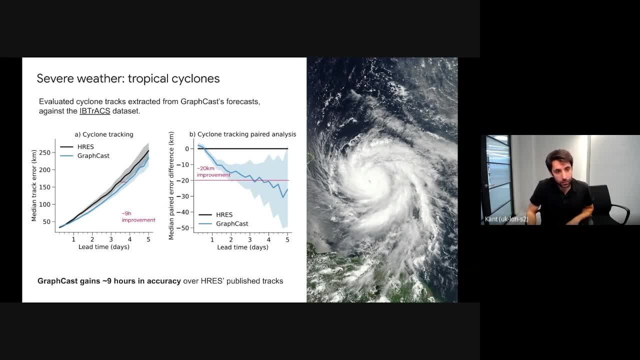 set Cool, Another one. So these nine hours and 20 kilometers, what do they mean? Yeah, Yeah, So, okay, So yeah, on the left, we see that. we see the median track error. We reported median on the main text because we found that a hard-coded tracker sometimes. 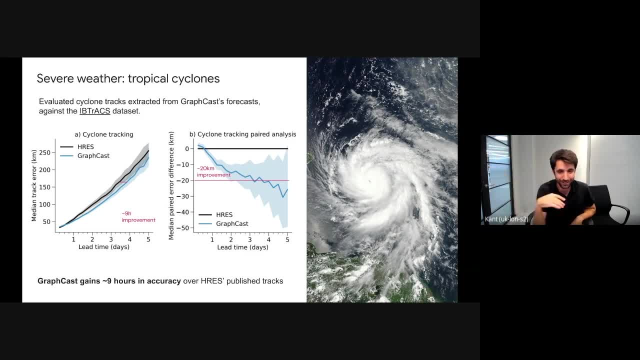 makes mistakes and just mistracks the true track predicted by our model, And so this was less sensitive to these outliers. but we also do better on mean, And what we see is that if you look at hres and graphcast, you see that the graphcast error is. 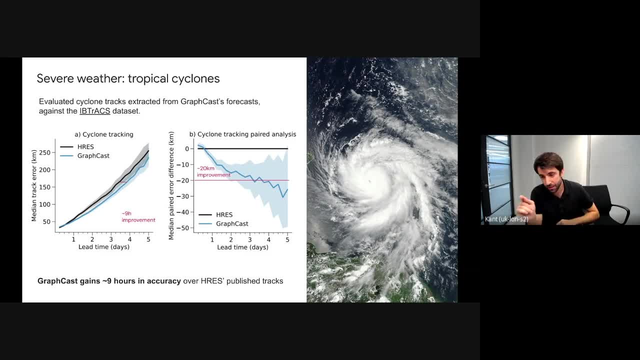 lower right. And what these nine hours mean is that we can essentially warn with the same level of accuracy as hres nine hours before, hres right, Because our error is the same as hres nine hours later. So we can warn with the same level of accuracy with nine hours more. 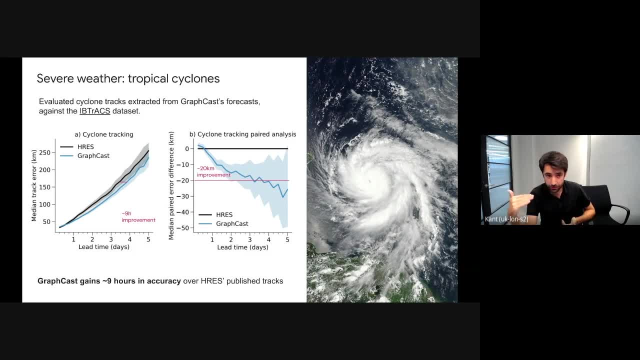 And on the plot on the right, we essentially look at kind of the vertical, vertical distance for a single lead time. how, how low, how much lower error we get with graphcast than with hres So we can say the location, the center of the hurricane. 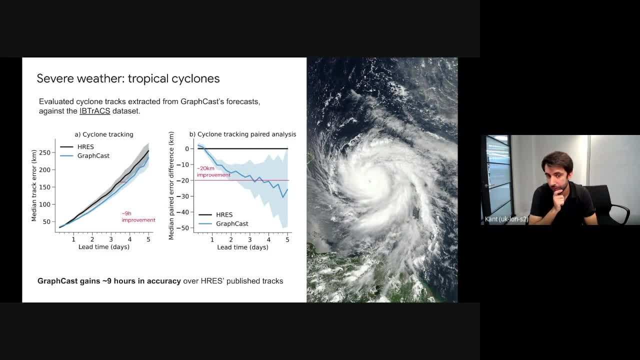 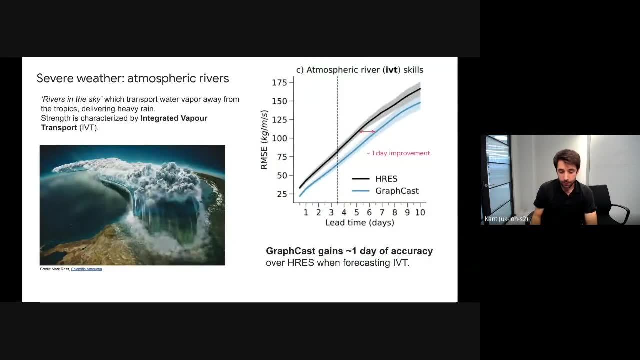 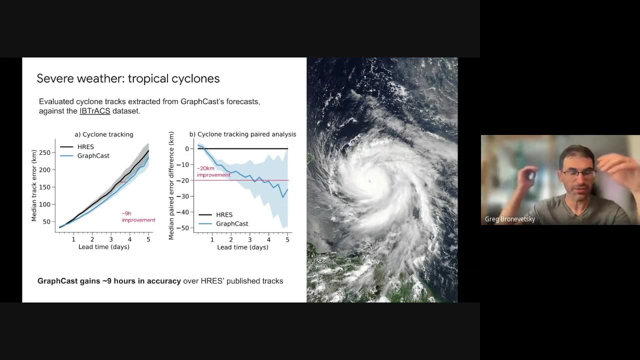 we can predict it with 20 kilometers better than hres. Did I answer your question? Yeah, Awesome, Yeah, Oh. and then one more thing. These are live things. So one challenge for dealing with any any weather data is that you have satellite sensors and ocean buoys. 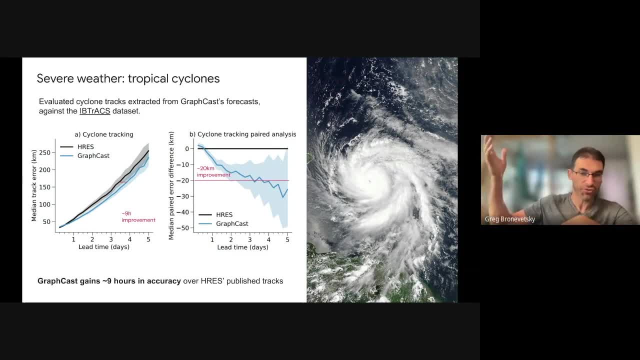 and whatnot. It takes a while for them to go up to central servers and then go into like a reanalysis, like grid, which you typically don't get in live And but your data set obviously is is reanalysis. So how did you bridge that gap in freshness of data? 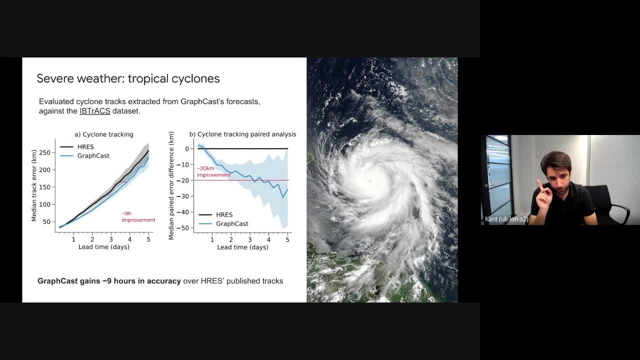 Yeah Yeah, That's a great question, So I'm going to talk about this in a lot more detail in in a few slides. That's number one. Number two is that even hres, so in practice, how it happens at. 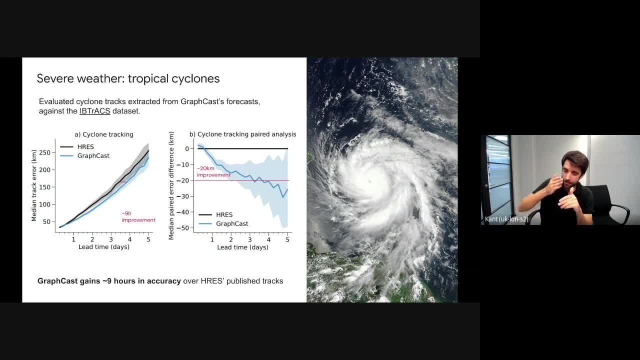 deployment time is that you do reanalysis, I think, for, like, you're constantly getting the sensors and then you actually do reanalysis and go back three hours into the past and then predict from three hours into the past. That's how weather prediction is done in practice. So you use the 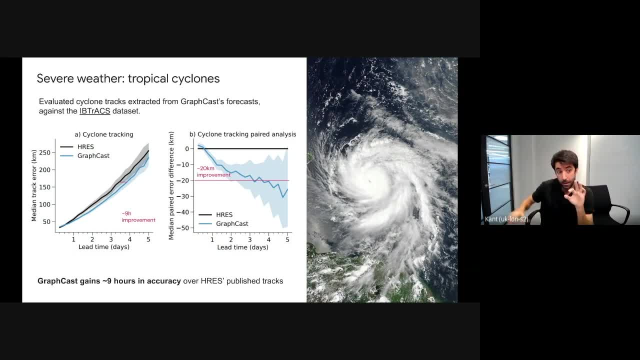 present to inform the model of three hours ago and then you predict from there These. there was a bit different, like the hour data set doesn't quite work with these three hours, And so we had to be very careful with that, And I'm going to talk about that in a little bit. Yeah, 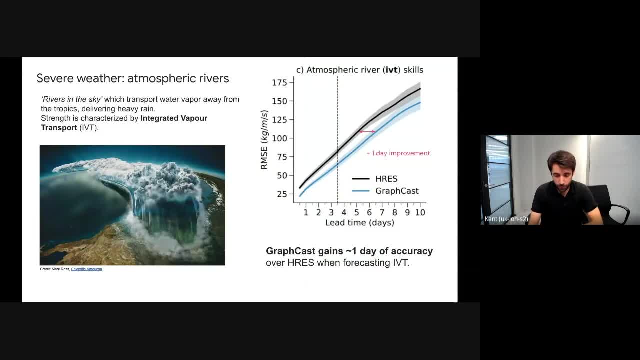 Excellent, Cool. We also looked into atmospheric rivers, which are a weather phenomenon that transport large amounts of weather vapor away from the tropics and can cause heavy rains. This is characterized by the integrated vapor transport, which we call IVT, which is something that can be. 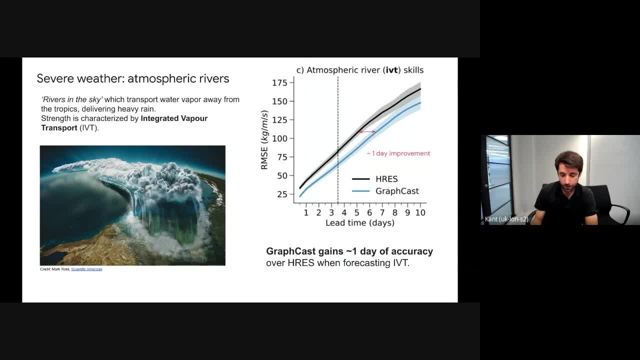 computed from the weather variables that GraphCast predicts, And we evaluated this over the US West Coast during the cold season, which is a season known for these atmospheric rivers, And we compared the performance. And we compared the performance of the atmospheric rivers to the weather variables. 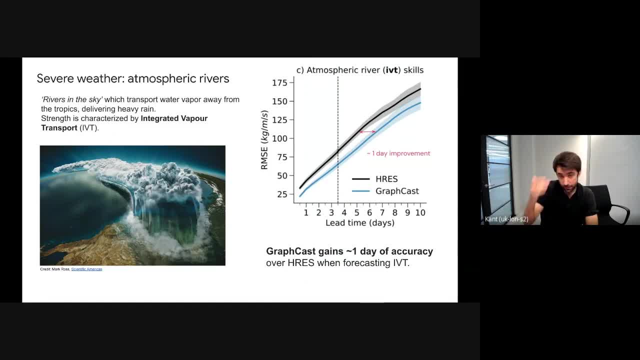 And we found that GraphCast. now it's not nine hours, it's one day of accuracy better in IVT, And note that this IVT we did not directly predict this. This is a nonlinear transformation of the weather variables that we do predict. 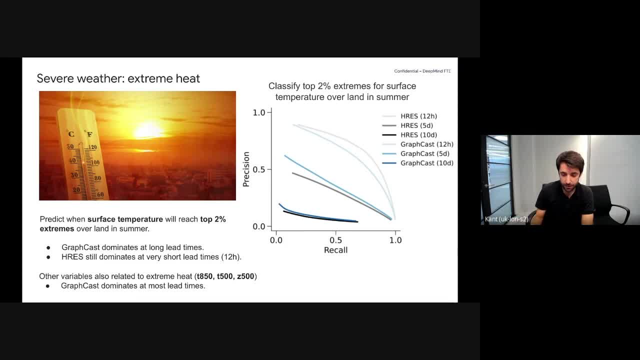 Finally, we studied extreme heat And in this slide we studied the capability of GraphCast to predict the top 2% surface temperatures using precision recall curves. And we do this as a function of lead times And that's why you have kind of three types of curves. 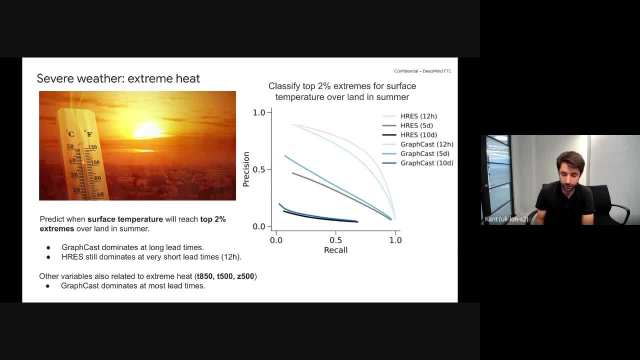 plotted in different shades of the color. We find that for long lead times, the GraphCast curve in blue is above the Atris curve in black, which indicates that GraphCast is better at the task, although Atris is still better at 12-hour predictions. This is not totally surprising. 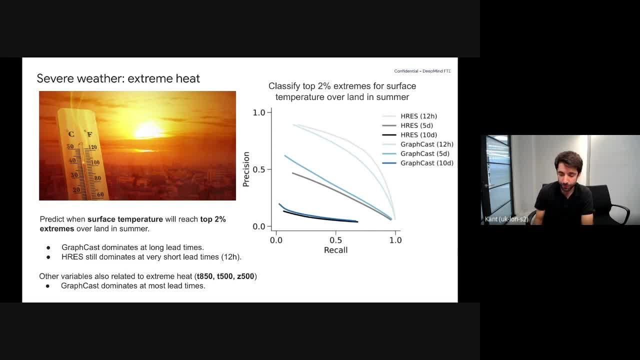 as this is consistent with the RMSE for surface temperature. However, it is still great to see that the gains in RMSE extend to extreme predictions, And in the paper Supplemental Material we show results for other variables And in the paper Supplemental Material we show results for: 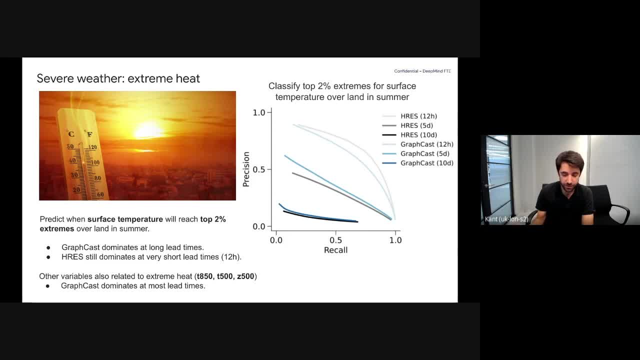 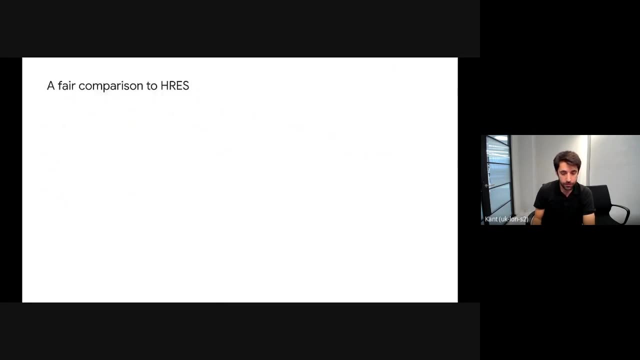 other variables relevant to extreme heat, as well as other metric regions, including extreme cold, of course, And in general we found that all these extreme phenomena tended to align pretty well with the RMSE results. So, going back to your question, a fair comparison against Atris, So one problem. 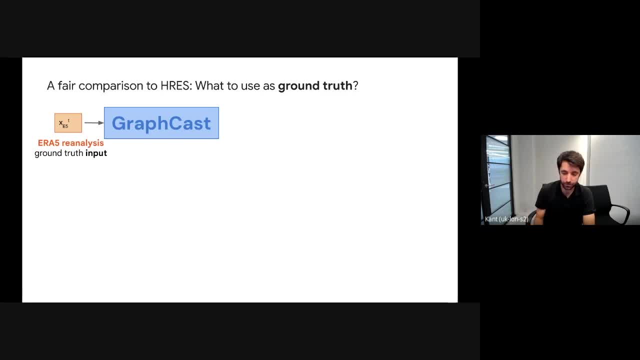 that we found is to decide against ground truth when computing metrics for each of the models And to understand why, let's go through what happens when we make a forecast with our model. So we take an initial state from ERA5 reanalysis, which is this: 40 years. 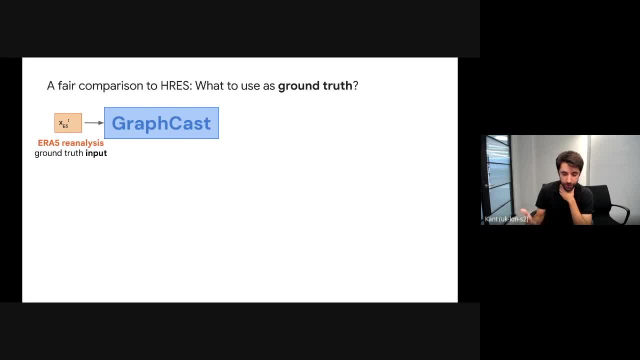 dataset and we feed it to GraphCast, And we do this because ERA5 is the largest dataset across all the years that we use for training, And so we of course want the biggest model for optimal performance, And this is going to produce a trajectory forecast. 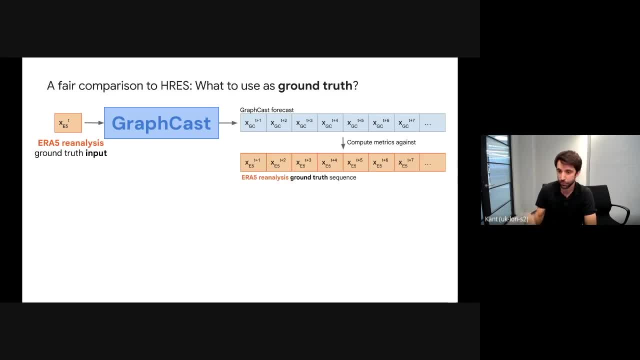 And then we compare it against the ERA5 reanalysis dataset to compute all the metrics result. So so far so good. However, we also want to evaluate Atris, but we don't have access to the Atris model, So what we do is we use forecasts that have been historically saved for each year. 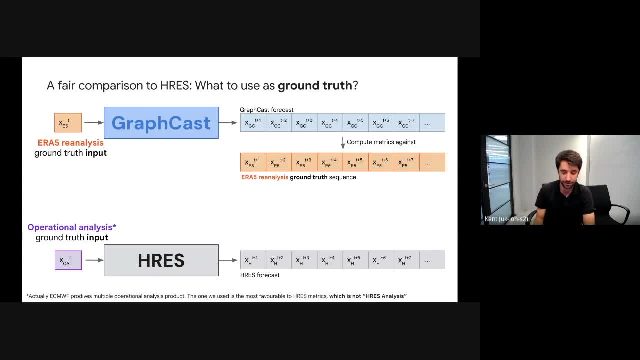 from a specific initialization and we call this operational analysis, And the problem is that the operational analysis and the ERA5 reanalysis they're very similar but they are actually not the same And this is thought out. but as a result, if you compare Atris forecast against 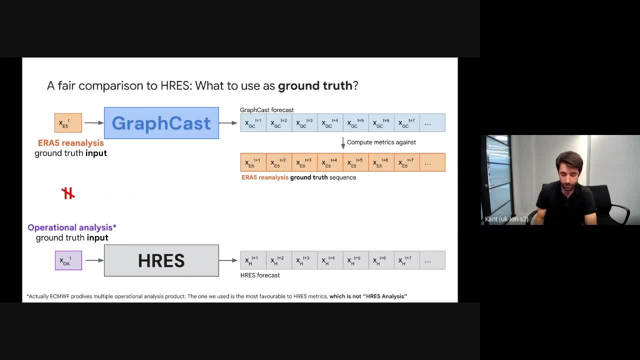 ERA5 reanalysis ground truth, you will find higher errors than expected. So after careful checks we essentially decided to compare against kind of this operational analysis itself. It makes essentially Atris look better than if we were to compare it in terms of ERA5.. 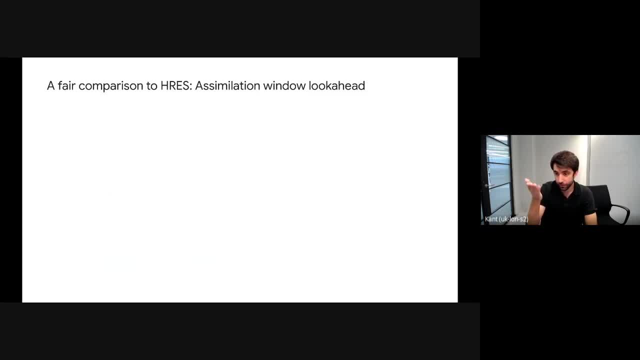 There's also another issue, which is this assimilation window that we were talking about on your question. Essentially, the intuition is that ERA5 reanalysis goes from nine to six, So you can see that for some horizon, some starting points. so what an assimilation window is is that we integrate all these raw sensing information. 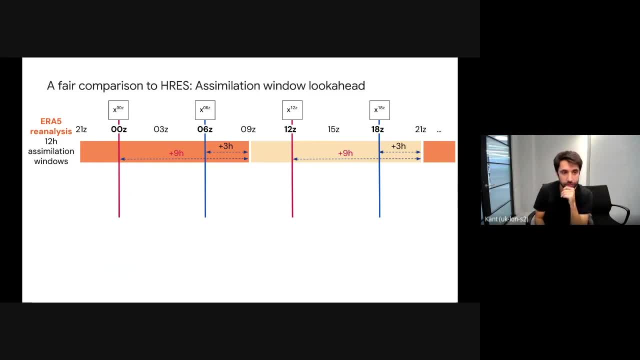 within one window to inform the weather states at zero hours and six hours, And so the zero hour starting point actually has some information leakage from nine hours into the future. So if you're not careful, models initialized with data five actually have a six hour advantage compared to the operational. 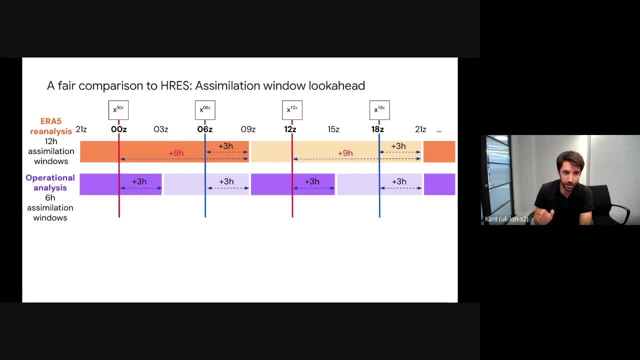 analysis which have different assimilation windows. operational analysis always has six hours assimilation windows and always kind of three hours looking three hours into the future, and that's why we decided to only show results that started at six hours, because six hours only has three hours into the future. and similarly we also only show uh results, uh, usually going 12 hours. 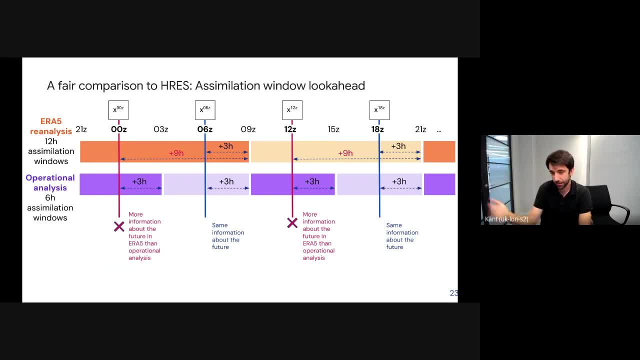 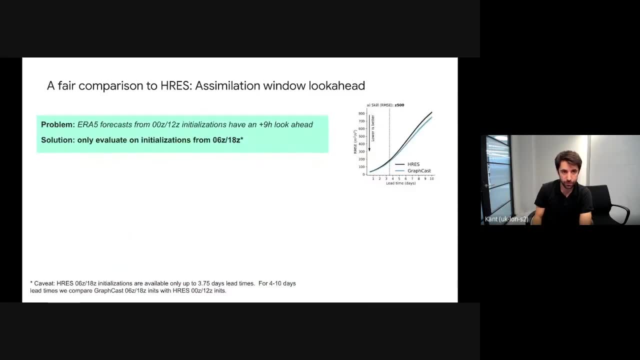 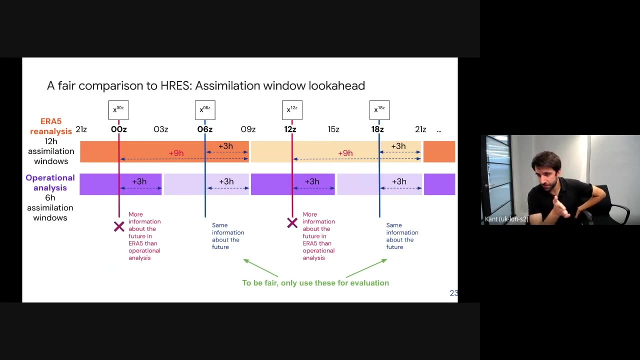 into the future. so multiples of 12, because then you're in the same point in the assimilation window. so we only use uh six hours and 18 hours. so okay, so you still have this leakage, but it's the same as uh exactly now we have. we have leakage, but like interest less and like any weather model. 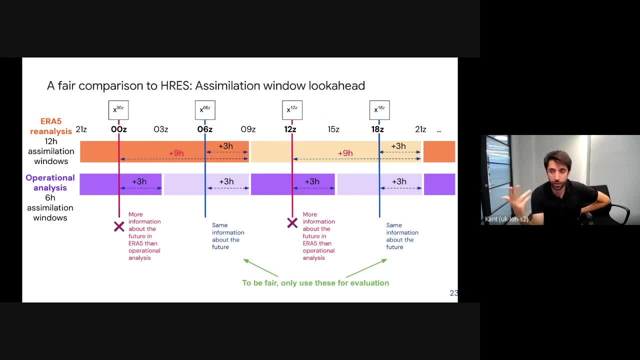 in used in in the real world they all have have three hour leakage and that's why they start from three in. in a deployment scenario they start from three hours into the first. so we have to be very careful in some papers initially, and even as initially we had made this mistake of comparing results on hrs at zero hours and 12 hours, which 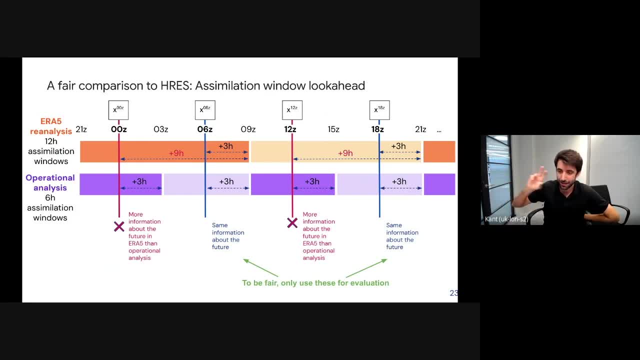 is kind of the most intuitive, but we found that actually we had the six, uh, six hours, uh, leakage bigger than hrs, and so, uh, fine, and i think we had actually this mistake in the first version of the paper, but the second version of the paper corrected this, or maybe i forgot, maybe we corrected even. 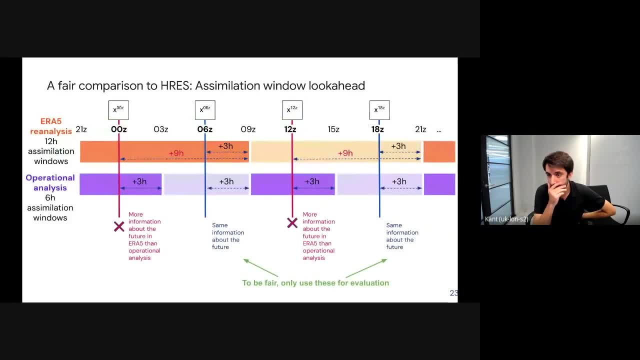 before the first version? um, yeah, i'm just curious. so when they um, let's say the operational analysis, if you take data three hours into the future and absorb it, assimilate it then, and then you start rolling forward again, you're going to re-predict essentially kind of what you trained on or what. 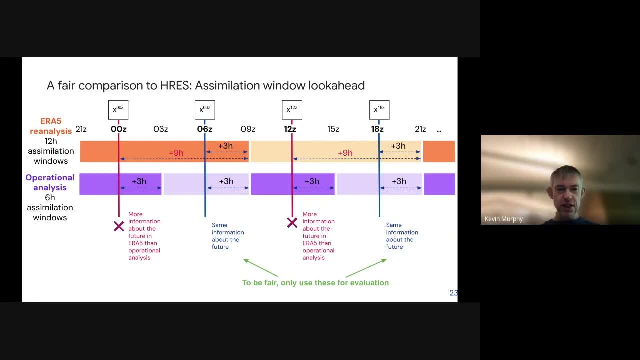 you conditioned on, and then, of course, you're going to make novel predictions. what's the description like when you re-predict back what you have already seen? that's like sort of internal validity, right? do people track that? yeah, yeah, yeah, that's a that's a great question. uh, we all, we actually found this, uh, this issue, and we found 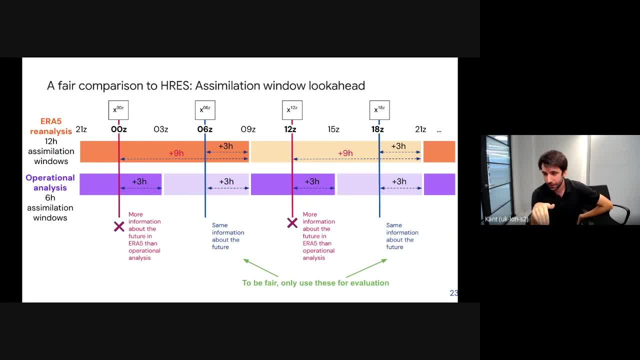 that it's actually much easier to predict within a simulation window than across the simulation window. as far as we know, when we were discussing with uh, the weather agency, and and other models, we were the first ones to kind of see this big being a big issue. i think people had kind of 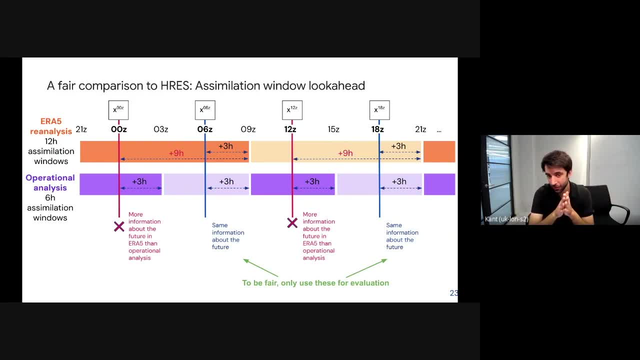 because the r5 reanalysis data set had not been used as a machine learning uh data set until last year. there were some of these issues literally had not been realized and and so, um yeah, people were not. we're reporting it as as if it was the same assimilation window, but we do see that the 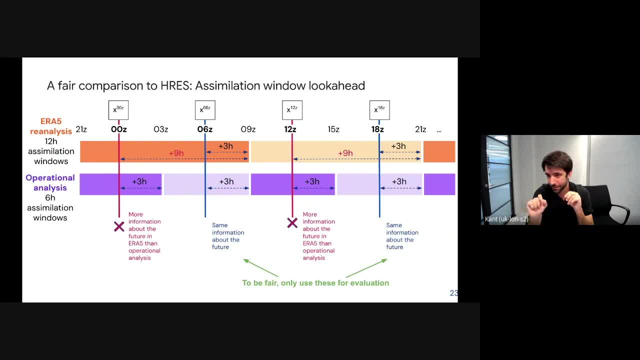 model is essentially learning two models: one within the simulation window, and it does very well that doesn't have zero error. uh, we think for two reasons: one, it's, it's not. it's not learning through interest, uh, not learning the true physics mode. and two, the the physics model also does not. 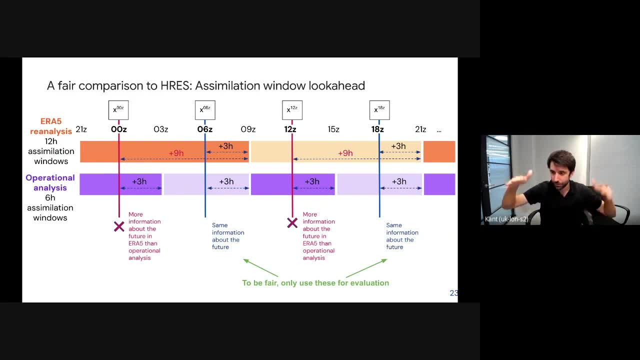 fully predict itself within the simulation window, because it has to, uh, come like, explain all this noisy sensing right, and then, once you cross the simulation window, you have, you have very high errors. well, not very high, but like comparatively very high errors. uh, yeah, yeah, thanks. so what would 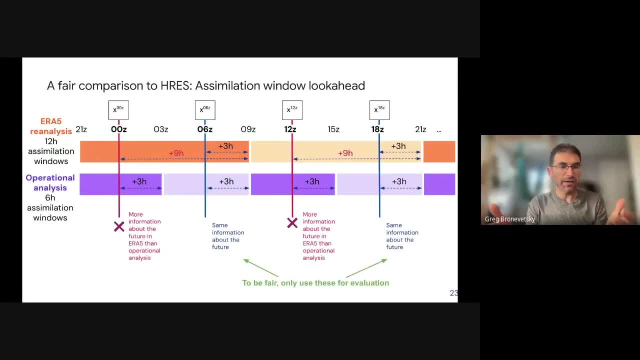 be the optimal way of doing this? because i mean, the setting you have is, uh, the raw data is not free to train a good model, so you use, uh, this reanalysis of some sort. what would the right, most favorable approach would be to have a different simulation policy and rerun the entire. 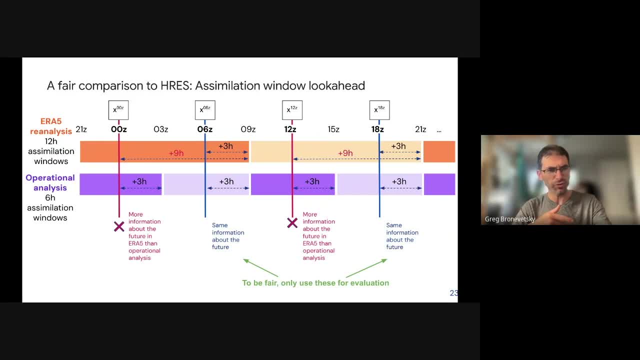 air five. would it be? um, would you want to have? i'm not sure. do you have ensembling for air five? would that help or hurt you? yeah, the good question. so i think there is a two answers to this one is: in the short term, the best thing to do is evaluate. take it a five, or at least what we've started doing is. 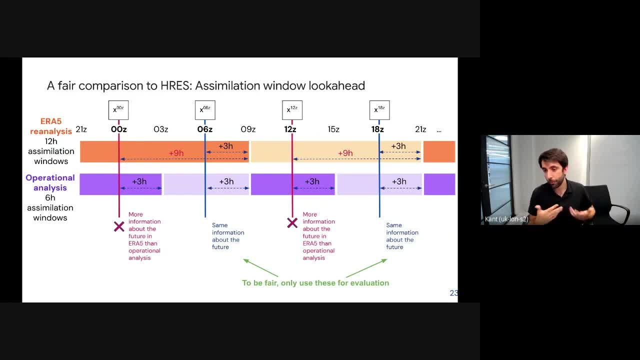 five, we fine-tune on this smaller, open, additional analysis data set and then we are comparing apples to apples and everyone's happy, um, and that's actually we've already deployed. so if one goes to this european weather agency, we can already see the graphcast models real running on, real, uh, real. 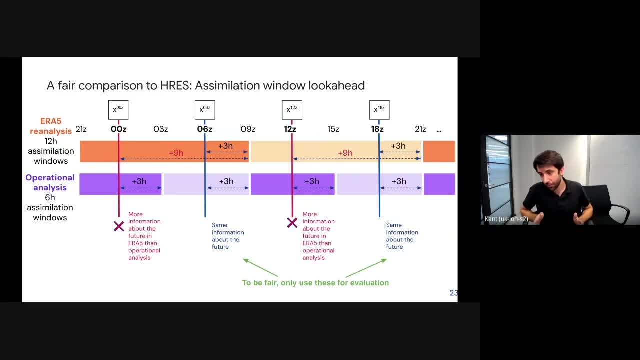 feet, uh, at real time, and that's how we actually did it. we trained with these four years in the area five, and then fine-tuned um. however, there is an even better thing to do, uh, which is kind of probably long, long term, which is just training on raw observations. right, machine learning doesn't. 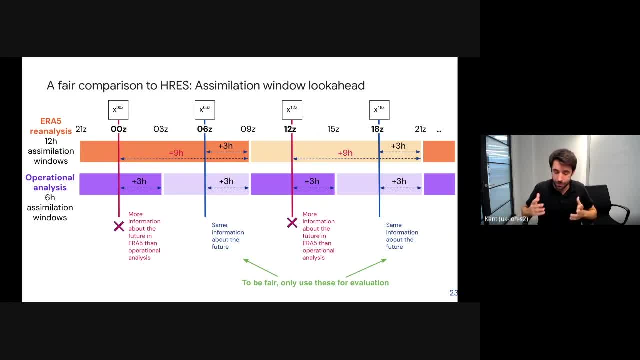 care about the type of of data that it runs. so we should just go to the rawest, uh, richest, source of information with just taking raw observations, which they will not be uniform in in time or space. so it's actually a very challenging research problem to work with this and also probably 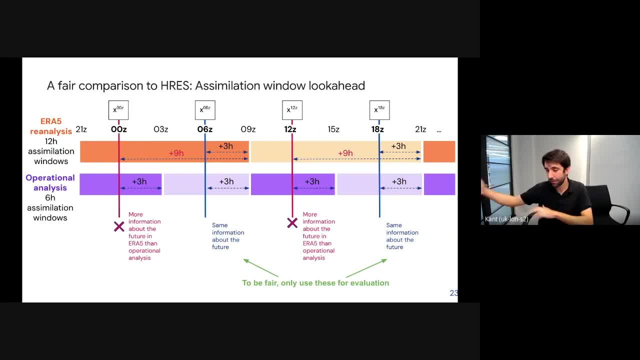 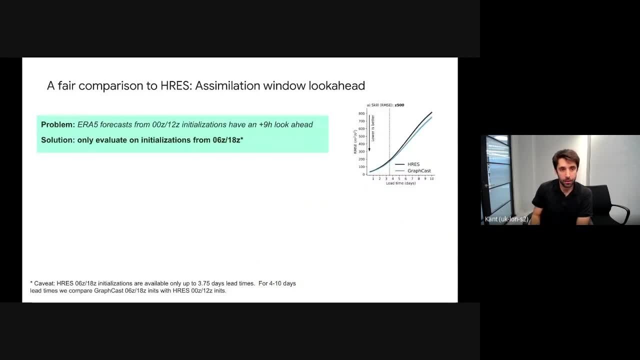 but it's probably what you want to do eventually- which the model then will have to learn to assimilate the data itself as well, but that's kind of more long term good, uh. so, in summary, uh, using this 6 am and 6 pm, uh was solving two problems. first, there are five. 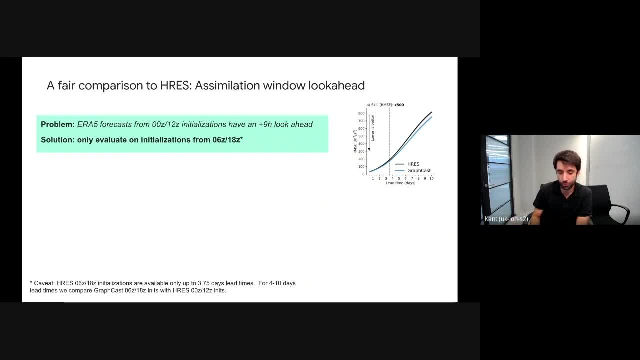 initializations at midnight and noon could potentially have a nine hour look ahead from a simulation, and this can give a could have given an advantage to graphcast. uh, so we only use 6 am and 6 pm, um, so one issue though, and that's why you had this kind of dashed line, is that address only? 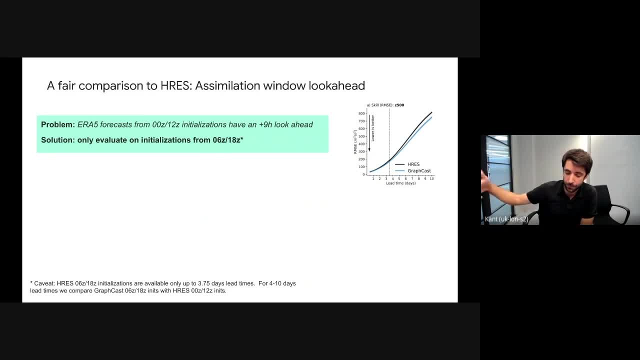 uh, the published address predictions only look um up to three days, three and a half days, sorry. so after this three and a half day curve we actually had to compare the six, uh am, 6 pm, uh, graphcast against 12 am and 12 pm. performance of interest, of course not predictions, but literally the rms. 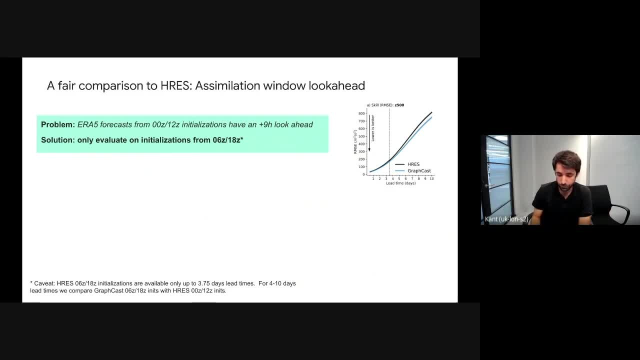 metrics of 12 am 12 pm against 6 am 6 pm, and so uh the. the second is kind of going back to uh kevin's point about, and it's easier to break within the same assimilation window rather than across the simulation window. so what we do? 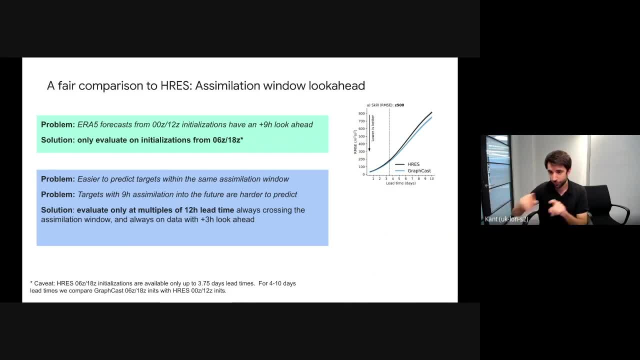 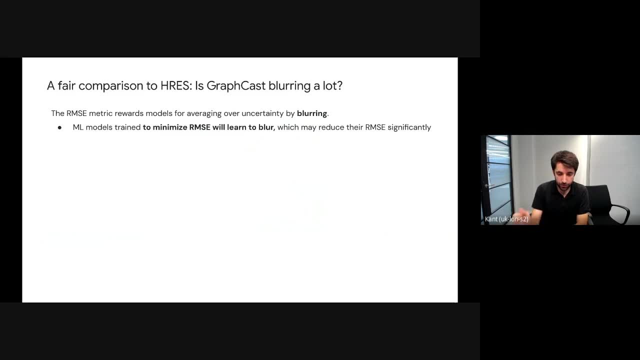 is actually only report errors every 12 hours, so that we're in the same point in the assimilation window, and we found this to be the most consistent. another disadvantage of the rmsc metrics is that, in general, rmsc rewards models that average over uncertainty, and, in fact, models like graphcast are often trained to minimize rmsc, which means that 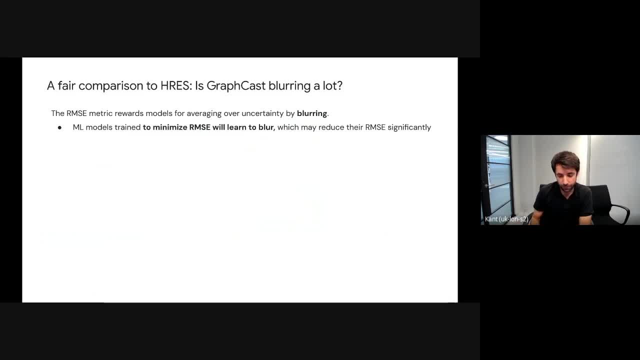 the training itself may teach the model to blur and, in fact, if we look at the power spectra of some of the variables, we see that, indeed, as we increase the forecast lead time, some of the power in the high frequency diminishes. so of course, uh, the question is whether it is possible that 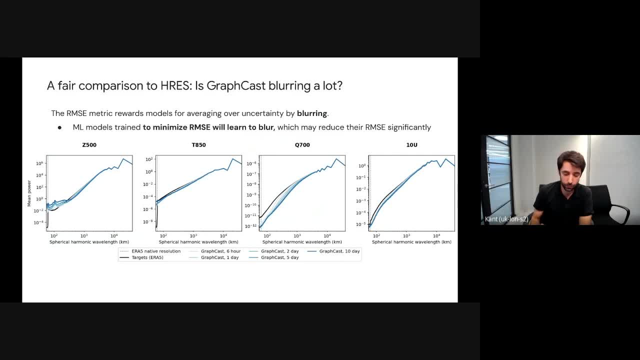 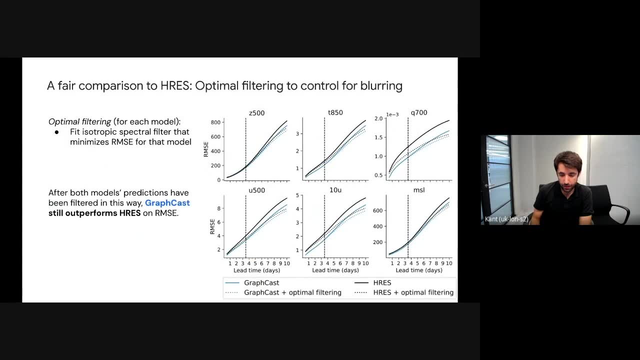 graphcast metrics are better simply because it blurs more when the hs, which is just trying to mimic the raw physics, uh, does not blur. and so to control for this, we recomputed the main metrics. but we now applied a post-processing step which adds a spatial filter to each of the models, allowing it to blur the outputs and the filters. 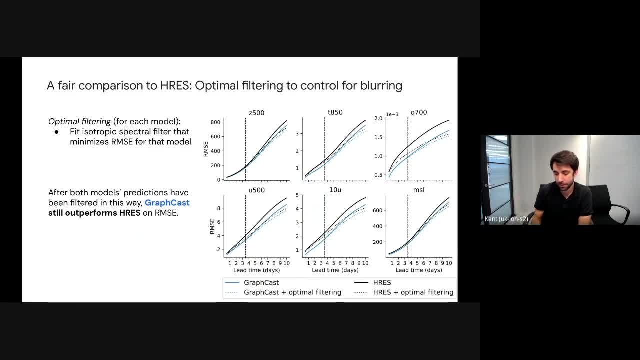 specialize for each model, each variable and each lead time, so that each filter allows to minimize our msc, and this is what we call in the paper optimal filtering. the plot on the right shows a dotted line, how the results of each model change as you apply this optimal filtering- and interestingly, not just address but actually also graphcast- can obtain a low end result. 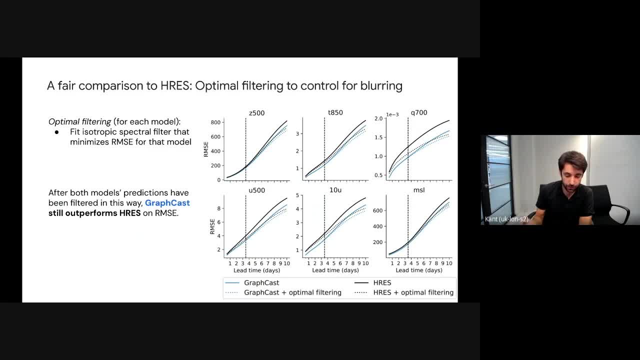 we see that graphcast still outperforms hs after this optimal filtering. so we must be learning a better weather uh model, not just um kind of checking this rms symmetry. i understand that. so you're essentially sharpening the generation from graphcast to make it you're. 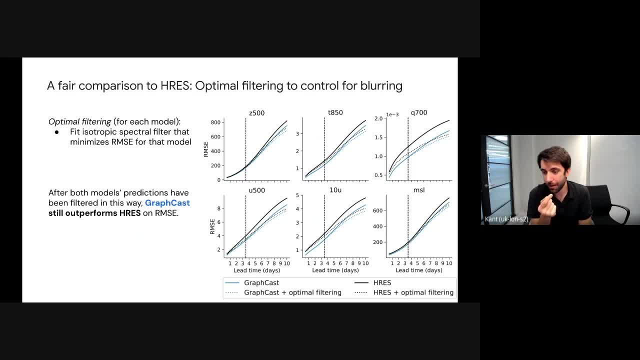 unblurring it with a post-processing token. no, no, the opposite, we are blurring it. so, because we know that blurring cheats the rms symmetric, we allow both graphcast and- uh, hrs to blur. oh, i see. so hrs has a free parameter for each variable to blur as much as it wants to minimize its error. exactly, exactly. 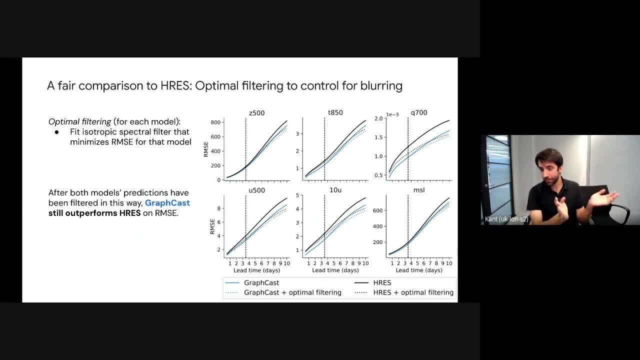 and we thought that that was the main thing. right, we wanted to allow hrs to to trick the rms symmetric, as because we thought graphcast probably was tricking the rms symmetric by blurring. so we thought let's keep hrs, that option as well. i see, okay, and then we also added this to graphcast: 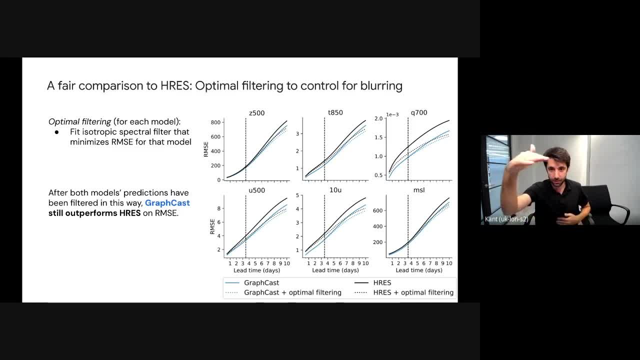 just in case we see that it helps. not as much, right, you can see that the the black line goes, uh, lower, much more than the blue line goes. and, in particular, one thing, let me see if it can be seen in these graphs: yes, uh, you can see that the dash line is only better than the blue line, like 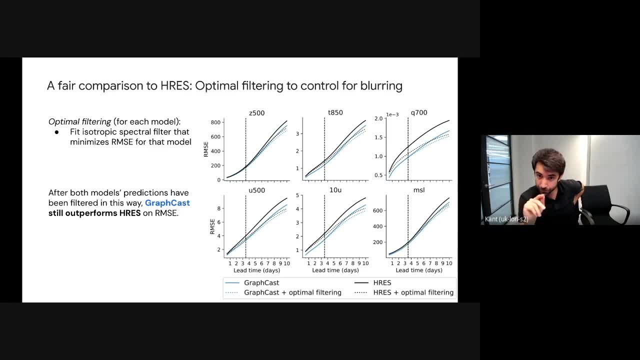 the dash blue line is only better than the non-dice line after, uh, about three days, which is our training objective. we only train up to two, up to three days and we hope that after training up to three days lead time, it generalizes up to 10 day performance and, as you can see, that blurring. 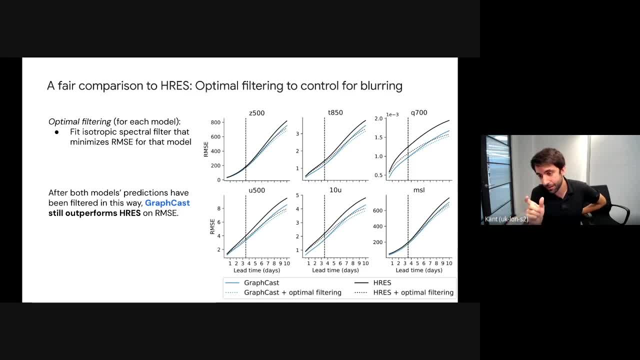 doesn't have be much with less than three days, and we think that's that's because, indeed, the model has learned to blur up to three days and then after this, optimal filtering actually helps to blur even more, um and fully kind of cheating as much as possible. these rms symmetric by blurring. 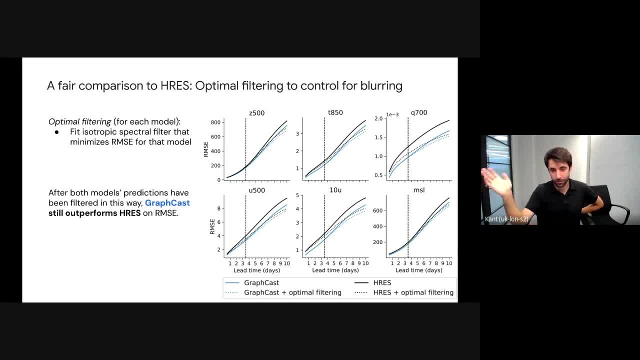 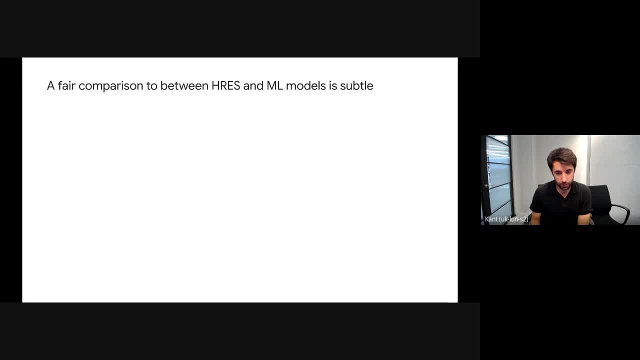 but we see that when you allow both models to blur as much as they want, uh, graphcast still does better predictions. yeah, thanks for the question. okay, so, uh, i guess that the takeaway is that the fair comparison, uh between operational models and ml models, train rfi- is pretty tricky, especially when models are initialized from different. 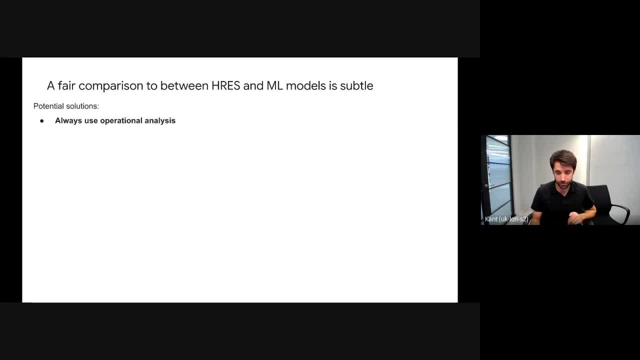 analysis and when models have different uh or of different nature, right? so one potential solution, which i believe it has become more common recently, as we were discussing before, is to evaluate the model on the operational setting graphcast rather than eta5. so in terms of potential solutions is i guess this is one of them, and so 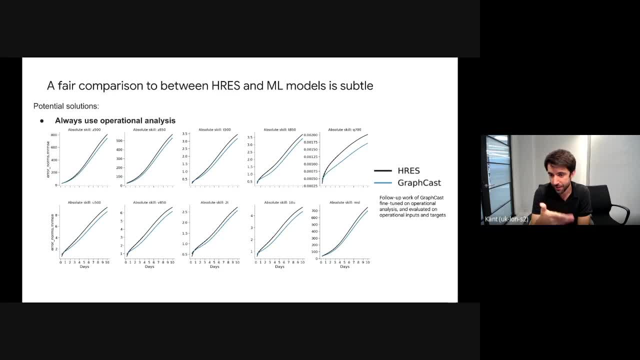 uh, this is the results on the operational analysis themselves after we fine-tuned uh. so after the the first uh archive, we published this, and so, um once, one suggestion is that hopefully the next version of era 5 will have this aligned assimilation windows that are closer to. 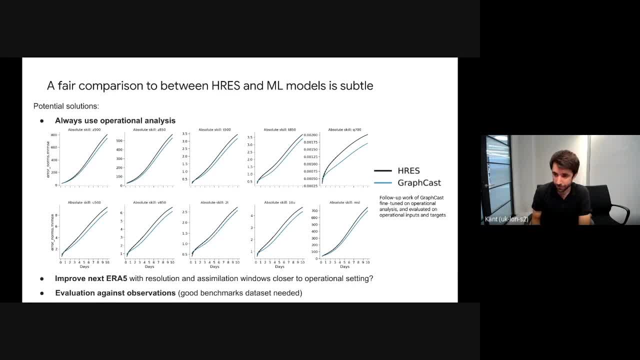 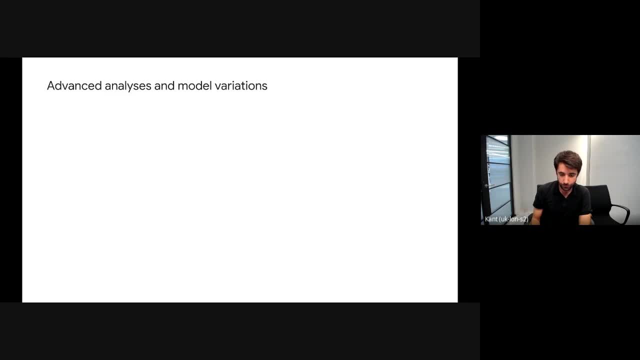 the operational setting. and, as i was saying before, uh to greg's question, uh, really, the best thing to do is is evaluate against observations. so so, just one thing that we i wanted to show is that we wanted to check the biases of our model in certain regions of the world. for instance, this animation shows where the model underestimates. 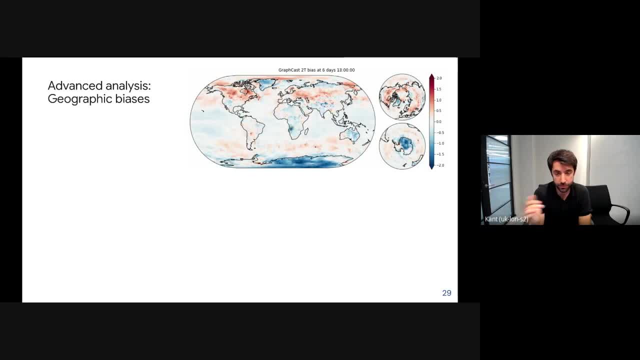 which you can see in blue, or overestimates in red the surface temperature, and it does so in different places on the earth and as the animation goes along, it's different forecast lead times. so if we look at this plot, we see that indeed the model has biases and that these biases 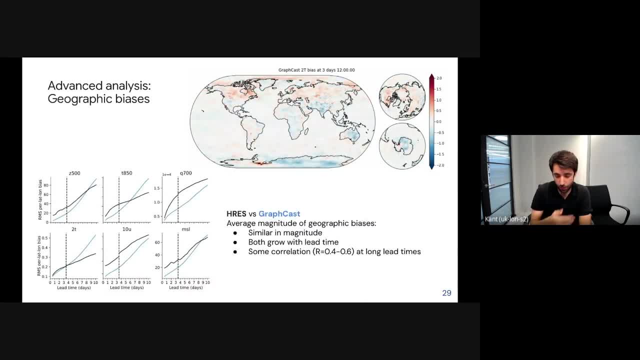 change with uh forecast lead time: uh. however, while this may seem like a lot of biases, actually these biases are comparable to the biases, that of aegis, in terms of magnitude, and they are. both of them grow in time, and we also actually found some relations between address and graphcast. 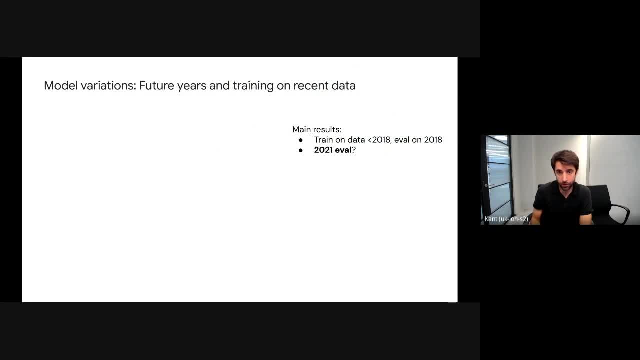 in terms of the biases cool. another thing that we did was training uh to make sure that like to to really the the effect of the database recency on on the model, and what we did was evaluating on 2021 and we tried training on uh up to 2018, which is our, our main model. so instead of we train up to 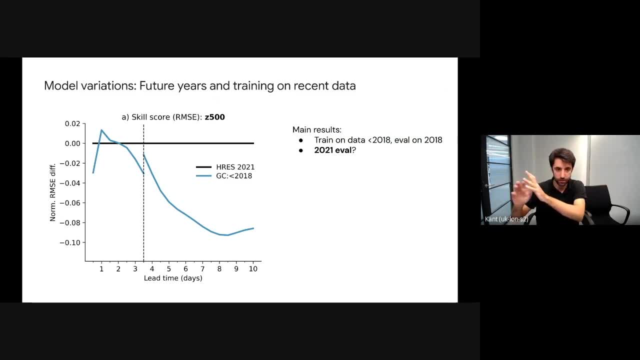 2017 and the main result is testing on 2018. but now we looked at 2021 and you can see that performance still better than interest, but not as much as one would hope. but as we add more recent data, performance keeps improving and improving. 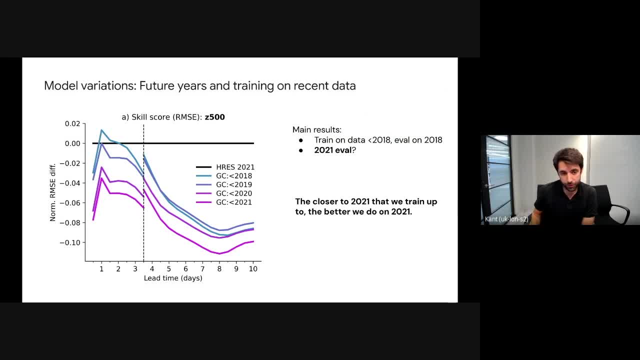 and so the closer we go to 2021, the better we do on 2021, which is nice to see. but we also indicates that there's probably some distribution shift. we don't know whether this is due to climate change or also a better uh sensing modalities. right, because the uh 500 assimilation data set. 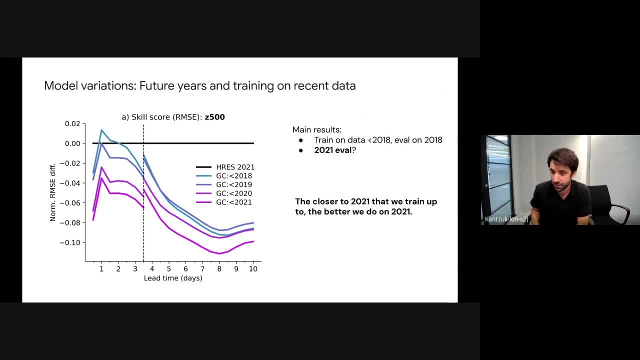 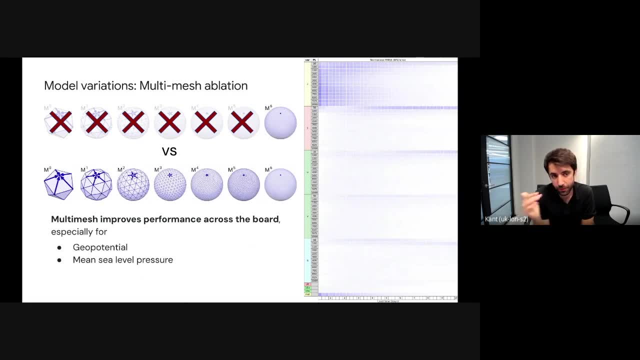 has been created with raw sensors, and these sensing monitors have been improving over time. another relation that we eat in our model is removing these long edges that we were saying before. um, maybe they were learning some, some non-physical uh parameters, and we see that in general they tend to help, especially on geopotential. 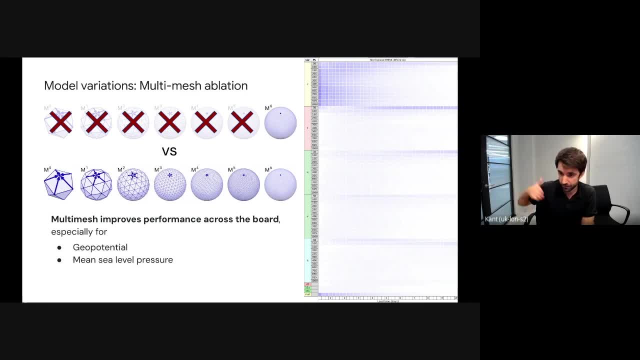 and and means level pressure, which are essentially the same, the same quantity at different levels of the atmosphere, and these are tend to be smoother fields. so we think that probably that's why uh having these long edge dependencies uh helps in both cases, but it seems to help across the board. 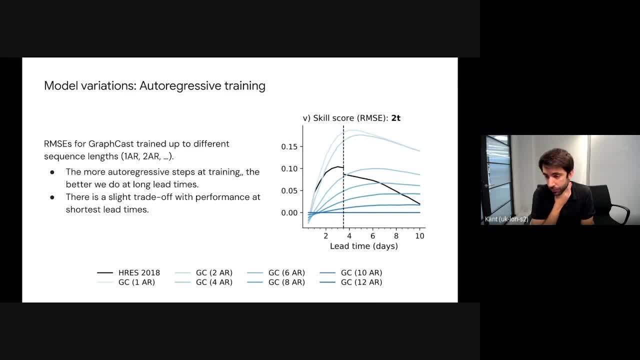 and finally, uh, we also looked at the effect of autoregressive training, right, so, uh, one, we have the option of just training to do well at six hours, or training the same model to do well at six hours and 12 hours, or, uh, training it up to 12 hours of the regressive step, and we see that this is essentially performing. 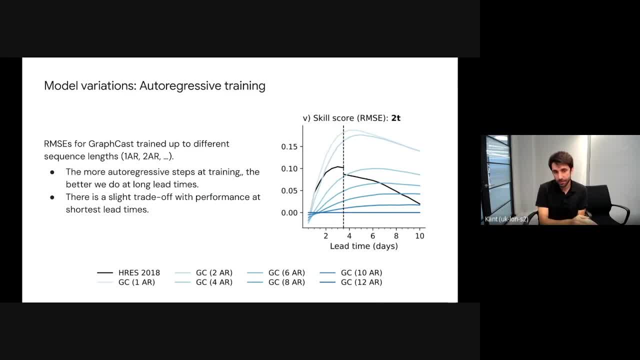 a trade-off. uh, so uh, the model when we only train into one autoregressive step is the best model at one of the regressive step, and as we increase the number of training steps, we're essentially shifting the curve and balancing um, doing better at longer lead times, uh, with doing worse at shorter. 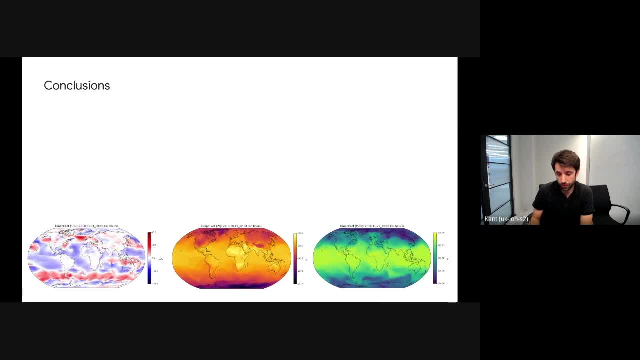 time frames. so the other one. we have the option of uh operating the graph as well, uh to do the same uh. so, in conclusion, uh the graph has output, outperforms entries, which is the best operational model. uh, in many ways we have seen how it does better in the typical rmsc metrics, but we have 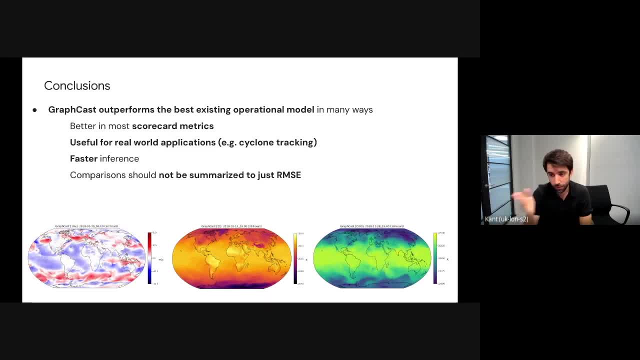 seen that also. this translates to better- uh, real applications. it's also worth noting that now inference just went down from one hour to one minute, which also allows us, if we wanted to, a single prediction. that would also be much cheaper to do, And we think that we have to be. 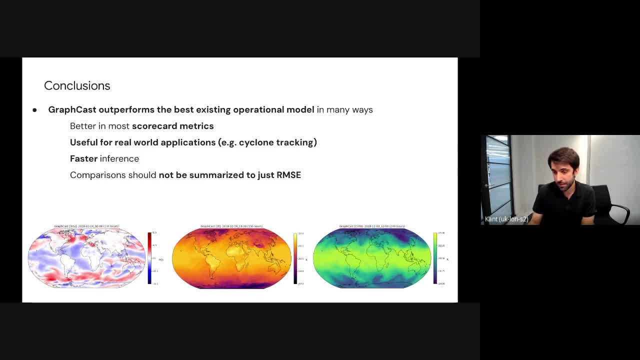 careful and make comparisons that not just apply to our MSC but real applications that benefit the end user. And the second conclusion is that deep learning weather models are probably here to stay, So last year and 2023 have been kind of key years where deep learning has started to. 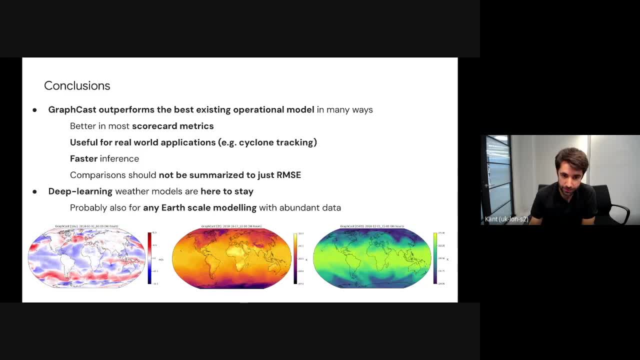 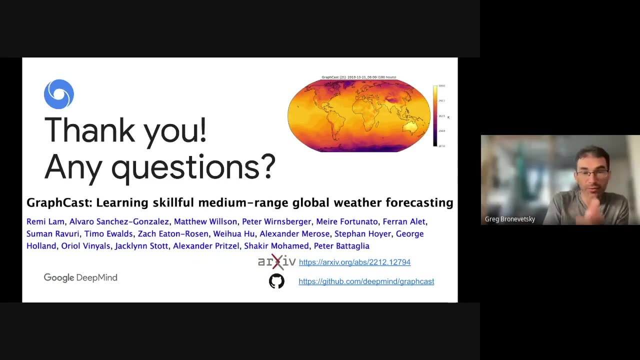 surpass numerical weather prediction And, as the data keeps increasing, any earth scale modeling using deep learning is going to outperform classic physics. And that's it. Thank you for your attention. Well, thank you very much. Are the questions in the column? 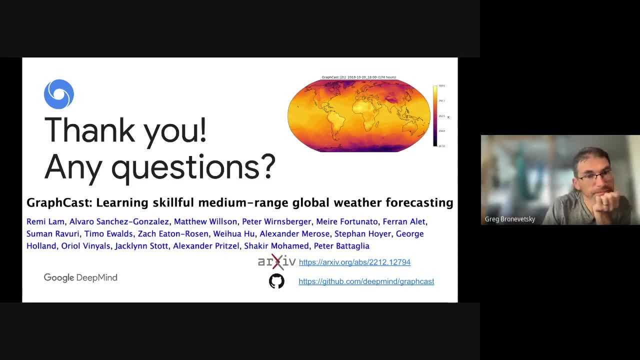 Well, okay, Oh yeah, Yuzheng, I have a question about: Have you ever heard about? Google has already released a weather bench- And what's the difference between the weather bench and this? And I see weather bench has also include this. 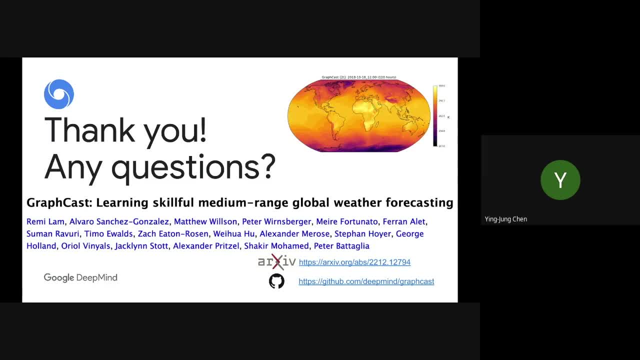 paper for GraphCast and also the PanGroove transformer weather model. And then, so what would be that you guys- because I know Google has been consolidated with DeepMind, So do you guys were like actually cooperate together, or just different types of model? 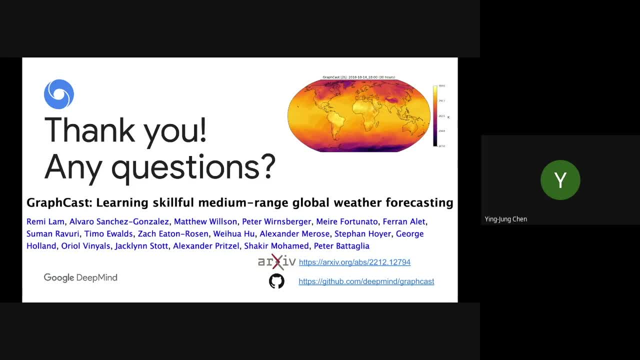 And what's the purpose? have two different types of model Because there are so many weather forecasts and and also NVIDIA has their weather forecast too. And then I just want to know the purpose, because I'm a hydrologist purpose, And there are so many and I'm not sure that weather forecast. 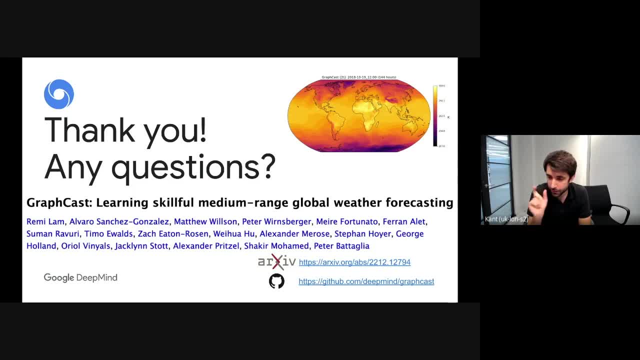 will help for hydrologists. Yeah, I didn't understand the last sentence, but in general, so there's two answers to your question. One is: what is weather bench and its relationship to GraphCast Weather bench, as kind of the name implies it's? it's more like you know. 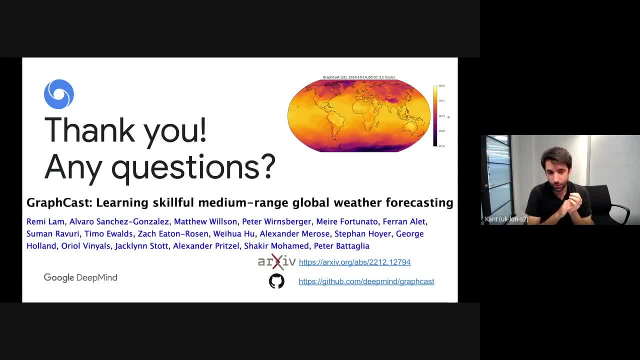 the, the benchmark than the methodology. So weather bench, I forgot if actually the well, there is some sharing between the others in in in our paper and weather bench. Actually I was not involved in weather bench but many of my colleagues were and essentially just think 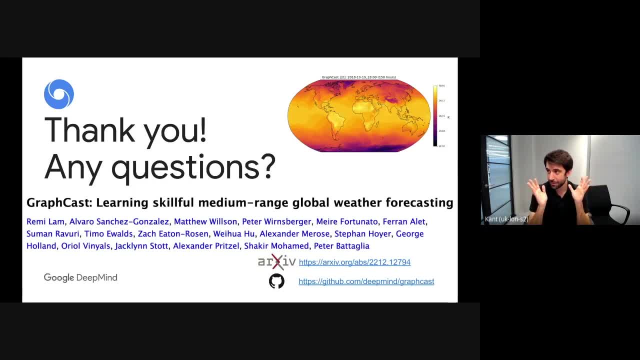 about it as the benchmark, So just as a standard platform to evaluate weather models. And, yeah, thanks for sharing the link. And weather bench two was, which is the link you shared, was recently open sourced to essentially just standardize weather prediction, because 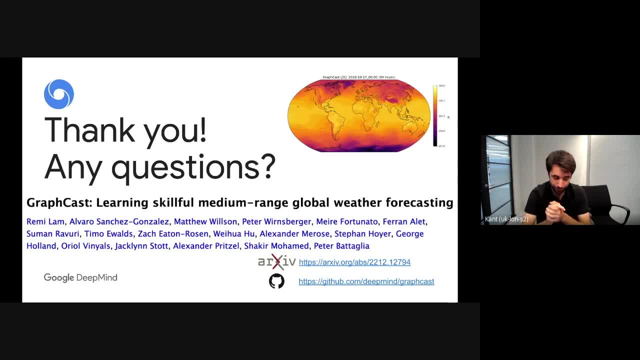 there are many things that one can do, can, can, there's many mistakes that one can do when evaluating weather models, and they make the right decisions, hopefully, and to make a standard for for the industry And actually the the creation of that benchmark itself kind of answers the. 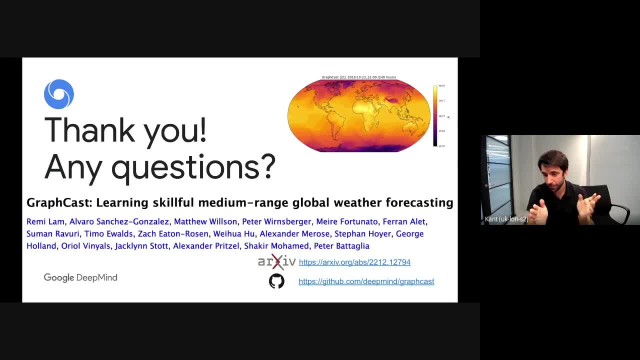 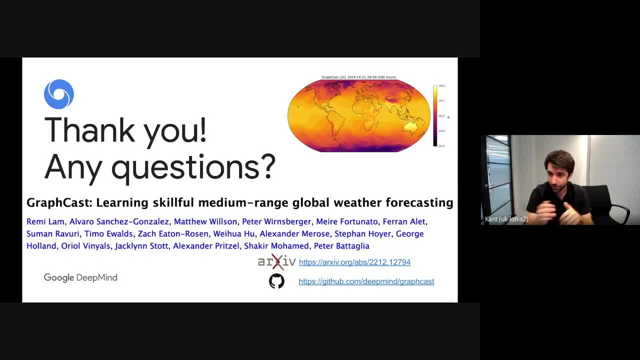 in research kind of this healthy competition across many different ideas, different teams. that's what makes progress go farther And we get on each other's ideas And we create some amount of independence to be able to explore different paths, Like, for instance, MVDA uses. 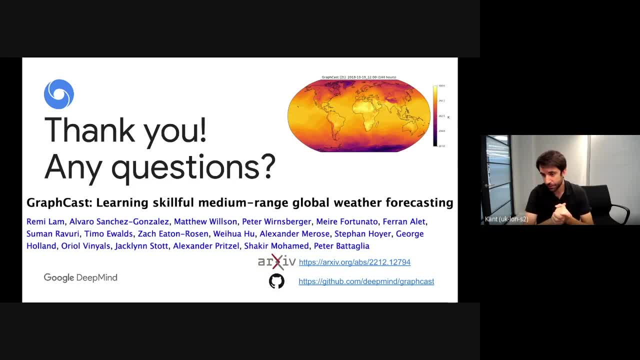 Fourier neural operators. Pangu was using transformers. we use graphing on networks. each of us is going to discover different things, And so we're going to build on each other's discoveries, and I think that's kind of the finishing touch. 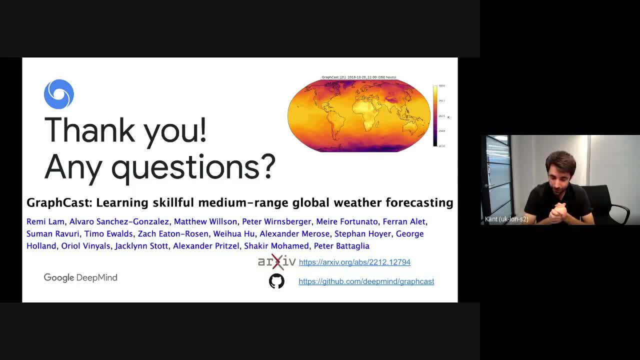 kind of the beauty of research and and kind of also, um, yeah, what enriches this unit? yeah, yeah, i'm just a follow-up to your answer. so i want to know, like, do you just just give you a case, like because you mentioned about atmosphere, river, so in case i always model, i predict, so how does the 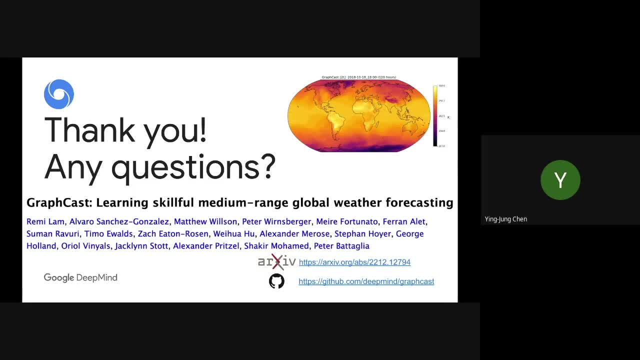 your model predict for atmosphere, river, land folding location or land folding? i mean, the ivt pass will be much more accurate than actually using the weather satellite measurement. i'm just curious. yeah, yeah, yeah, i i'm not an expert in this. uh, i think, remy lam, if you want to uh. 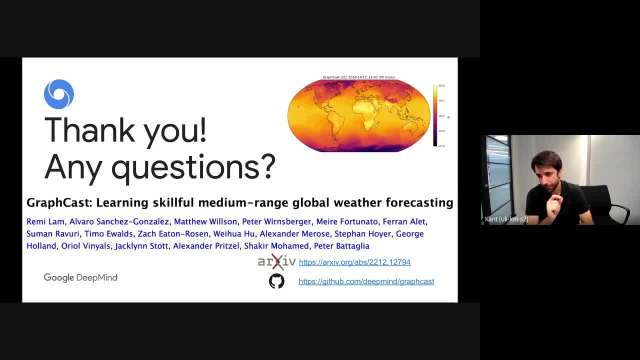 send him a message that he was actually the one that did the atmospheric, uh, reverse experiment. but as far as i remember, the atmospheric reverse is literally um a formula involving a few of the variables for every, for a few grids. so we have a few grid points in in. 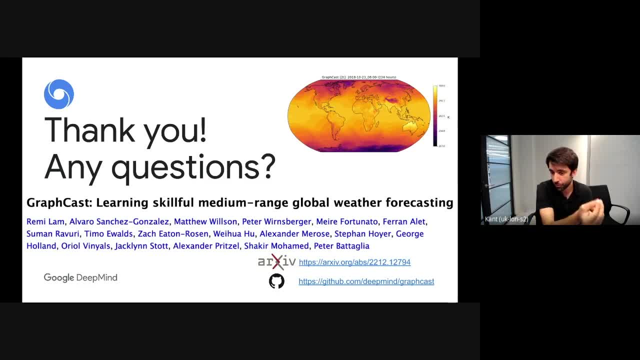 in our evaluation and we literally apply that formula both to the through weather, as well as our predictions, as well as addresses predictions, and we literally compare those numbers: uh, which one is closer to that? i don't think we have paths in the, in the, in the atmosphere or anything like. 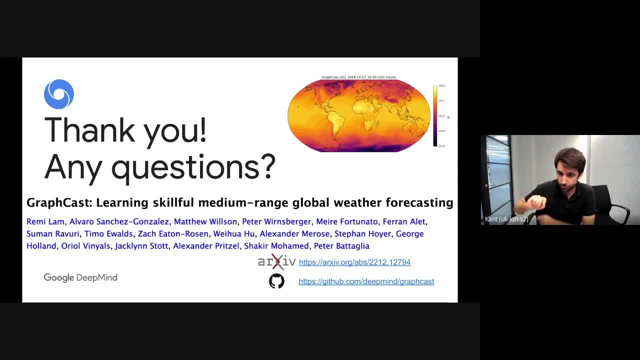 this. it's not like cyclone tracking. i believe it's literally predicting uh, specific quantity, which i forgot exactly what it was. i think it's what we call ivg, if i remember correct. but yeah, that's right. yeah, yeah, that's how i did in my phd. yeah, yeah. 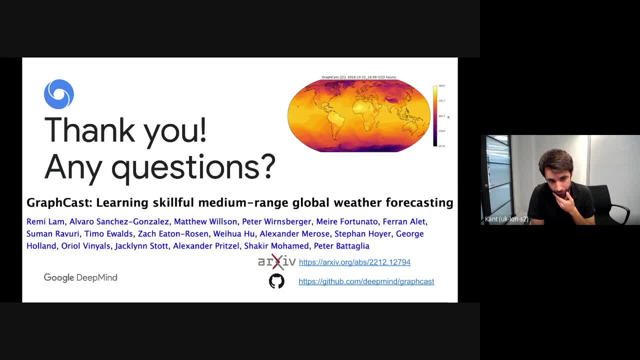 one, yeah, one one thing. i guess this is a good show of of the fact that the machine learning community it's a we we know very little about weather. uh, we try to learn as much weather as possible and and kind of we think that that, uh, we try to be as careful as possible. 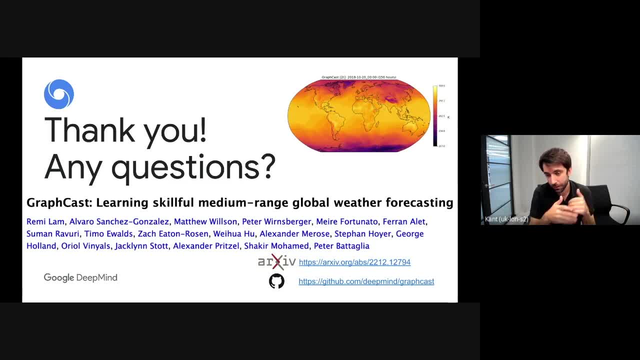 and as responsible as possible in our evaluation, but we've also been in talks with uh weather experts to make sure that our- our predictions are consistent and meaningful as possible. uh, and so, yeah, any input that you have uh in particular in this field if it's your expertise. 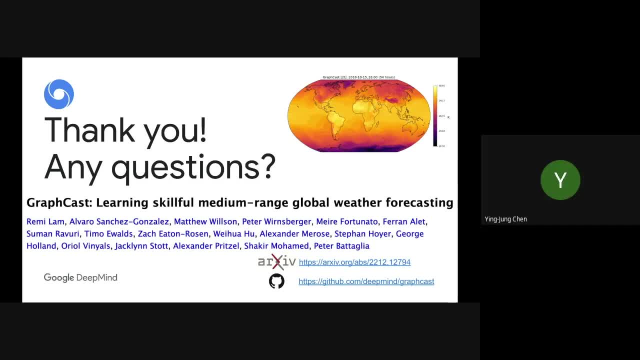 uh, if you message remy, i'm sure he'll be very glad to thank you. okay, one more thing. i'll just leave you a link to freddie cancer, who i just realized is a google now, uh, who does hydrology. so he's done lsdms for hydrology and, as far as i understand, like hooking up different river systems. 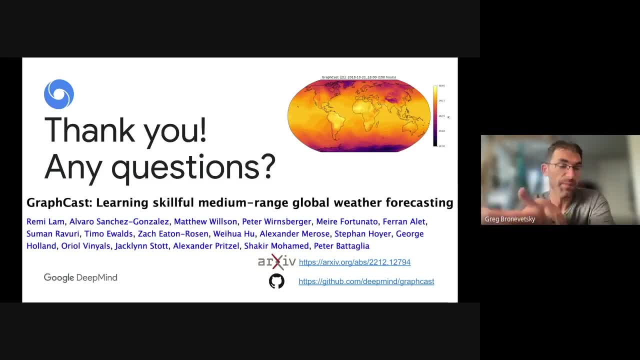 and he's done pretty well compared to you know, physics inspired hydrological models, so that's another interesting approach. sure, sure, thank you, and raj, yeah, oh hi, uh, this was great. uh, i think my question is more as a weather enthusiast or like a hobbyist. if, if i want to do a crawl walk around on your model, do you have some tips or? 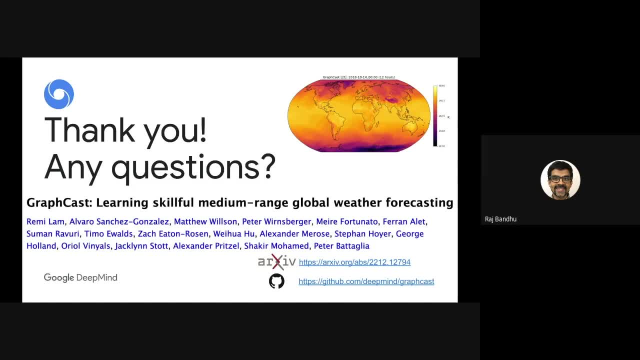 something like pointers that we can use just to have it more on trying to stand that up, just to you know, do it like like your, i'm my own, like local model for where i live and also i i was just wondering if you had some tips or some pointer or something like document you can point to. yeah, 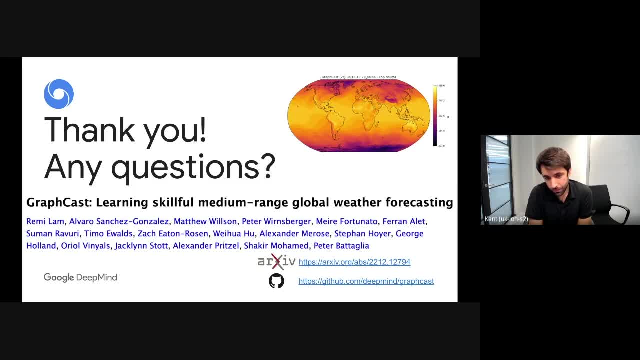 as time for time. yeah, yeah, i would recommend we we get kind of the two links that are on the slide. in particular, we have all the code for uh available on github. i don't think we have code for training. but again, if you're saying more like an emphasis perspective, training is super expensive, but 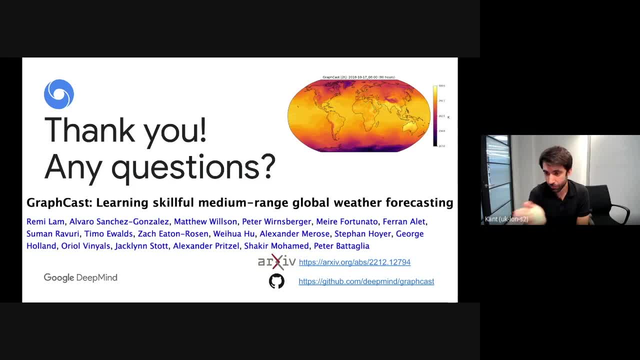 literally running the evaluation, like running the, the module prodiction is, it's relatively cheap, can be done with a with a regular gpu or also starting with a two to the. so sorry, uh, let me like with a smaller monitor and be like: well, that's really valid also, it, it, Yay, and you all have kind of fuckin mala interrupted me with all those if you take exams here. so here's. 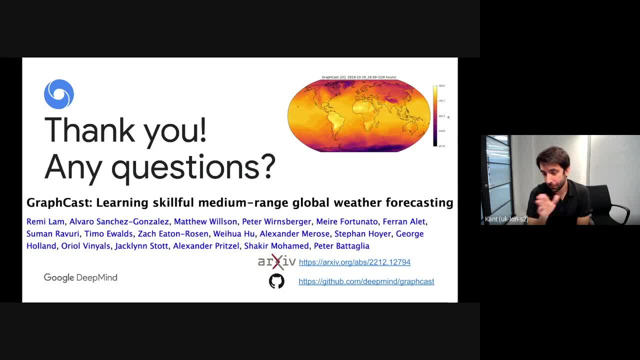 it's also part of the feedback that i had. i won't say it's been kind of awesome in getting people to get into these' smaller model. i think we also open source the smaller model that runs at lower resolution. that would also be a good example. and then another thing i forgot- if he has already published the 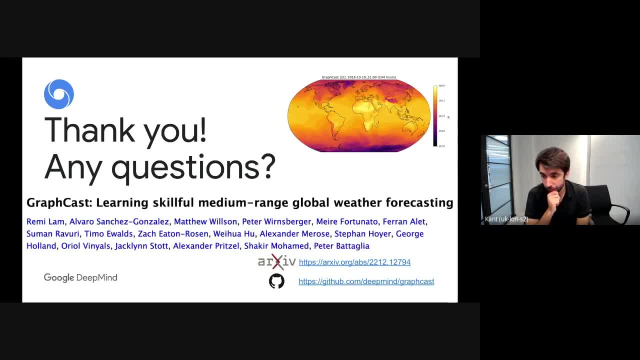 paper. but, uh, there was a recent large-scale deep learning bond conference where, uh, there was a pg student that used ideas from graphcast to run a local model- and also very cool, and both ideas from graphcast and graphcast predictions, i believe. so to combine it with a higher resolution model. 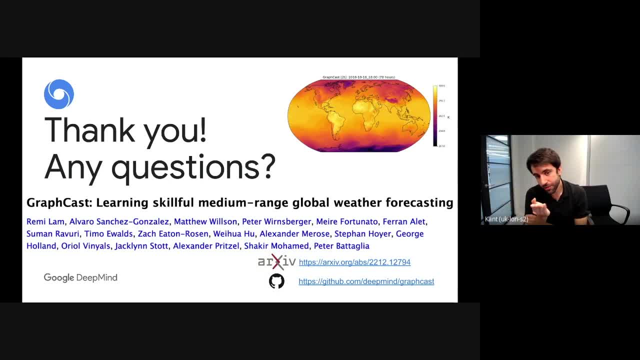 that was local and the intuition is that our resolution is still not the the resolution that one would get on your phone. so if you get your predictions on your phone, you you're using a higher resolution model, but how it works in practice is that it's informed by a lower. 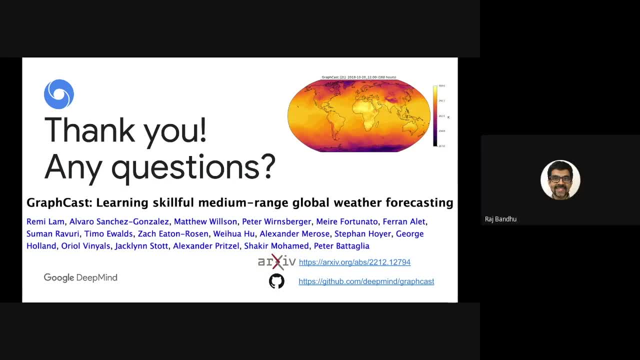 resolution global model, like like ours. oh, awesome, that is great, awesome. thank you so much, appreciate it. and performance wise, so that's probably a big deal. uh, in terms of how do you feel to compare the performance because you have? you're already based on errors, that's been already done uh. 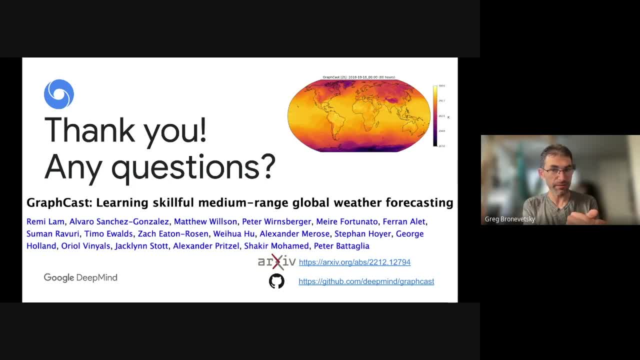 but, uh, the alternate models, how long do they typically take and like for a given prediction? yeah, if i remember correctly, uh, i think it's on the order of one hour, like. um, it's definitely much more than one minute, which is roughly what our predictions, and that's that's kind of the one. 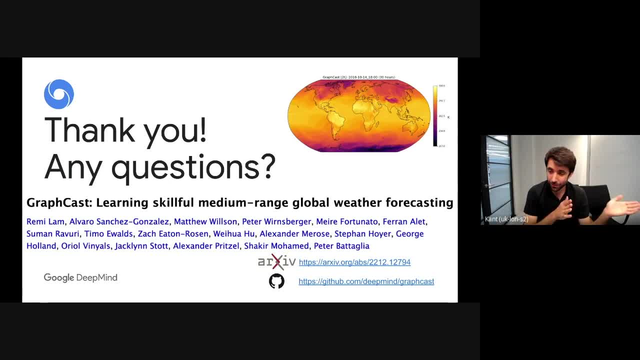 of the big advantages that ml brings to the table. that's actually, if you look at some of the papers, uh, from one year, two years ago. that's how they were justifying. they were worse than than uh weather models, but they were much faster. now we have both faster and better, so so that's uh. 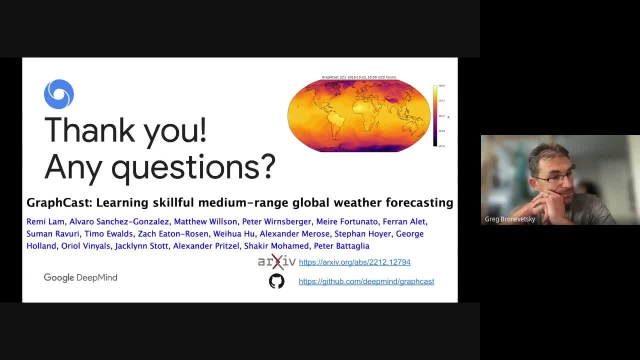 very good. and in terms of training, how long does that take? no, in terms of training, it's expensive. so we have about three weeks, uh, three weeks and three days, i guess, so 24 days, um, but it's, it's hopefully amortized, yeah, so one thing that's interesting about weather models is that 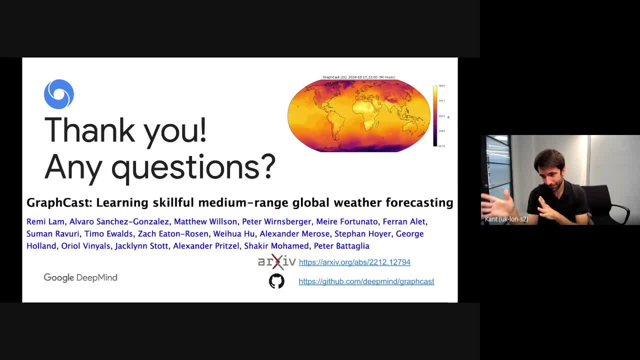 the training cost is bigger than the test cost, which is not often the case for many, uh many ml models. do you have any notions? he said 3d gpus and versus 10k cpus. is there a scale comparison between those two, i think? i think it's probably cheaper in our front, uh. 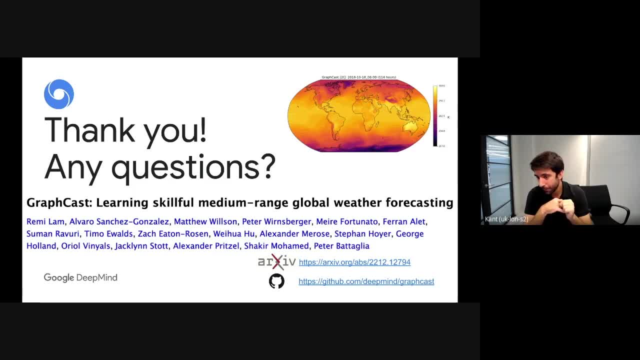 i'm pretty sure it's cheaper in our front, uh, and actually. but one interesting thing is that these weather agencies now have to shift some of their compute to to gpus because, uh, their clusters have been cpu based, um, so, but i think the call, the compute cost is much lower now. 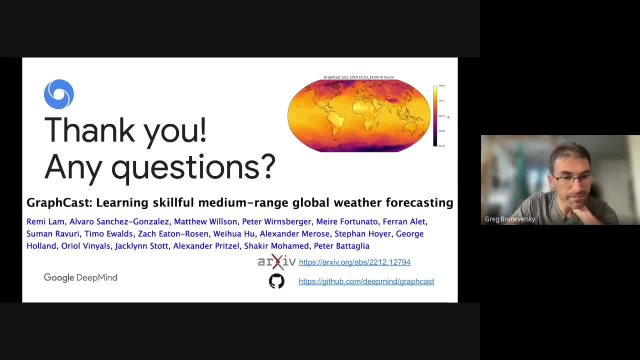 which is good for the field, right? yeah, kevin. yeah you, you mentioned um ensembles earlier, like, since you're already hooked into ecmwf, um, they have an ensemble forecast. could they not just take the initial conditions and run your graphcast code 60 times and you know you'd fill? 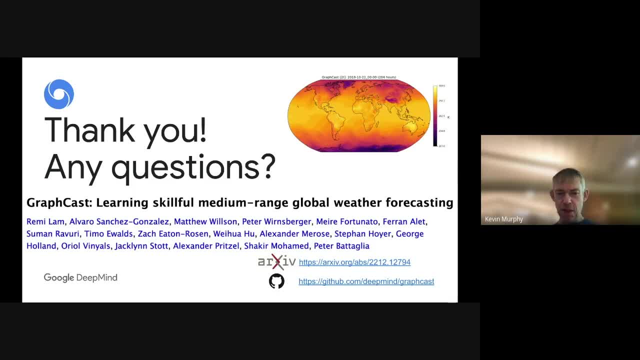 an hour. right, how? what? that seems conceptually straightforward. is it just an engineering task, or is there open problems there? no, no, we've done that internally. uh, and yeah, it's, it's good, it gives good results. uh, yeah, we haven't published this yet, but it can be done because 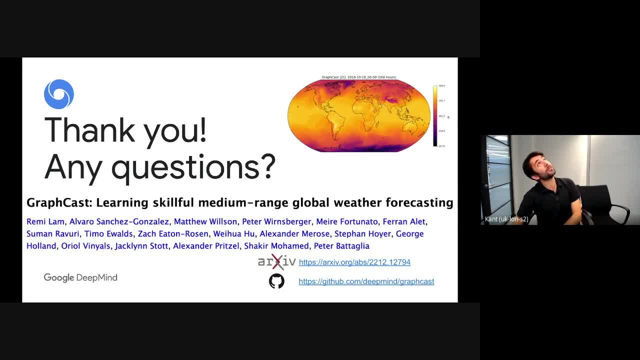 we've done it. sorry, i forgot, so let me just make sure i answer you properly. uh, sorry, we haven't hooked up, but we've done essentially something very similar of essentially perturbing the initial conditions and evaluating this, and it actually worked great. so just to um complete. 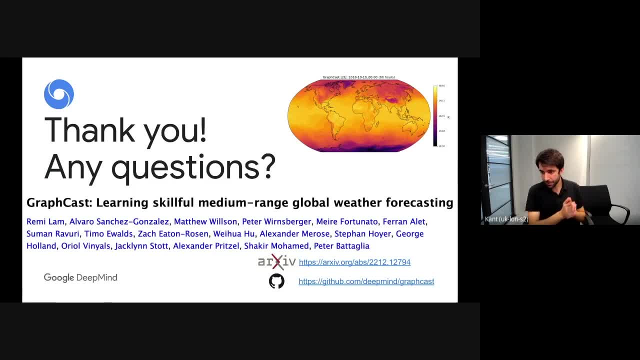 the answer? uh, we, we here. we say that we're better than the best deterministic model, which is, uh, what ecmwf calls hrs. but, as you were alluding to, you can perturb initial conditions. run it 50 times average the results. that gives better performance than the model we compared, against which this is. 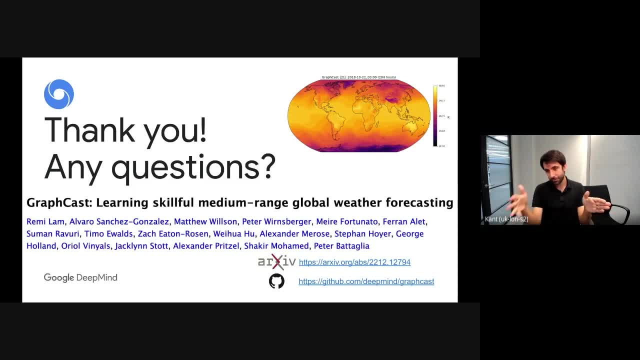 called ens. but of course, we can do the same to our model, perturb it and average it, and that gives even better performance and we think that this is probably better than ens. uh, we have to make sure that, uh, we like, like, internally, we think that it's better, but we- i don't want to make this- 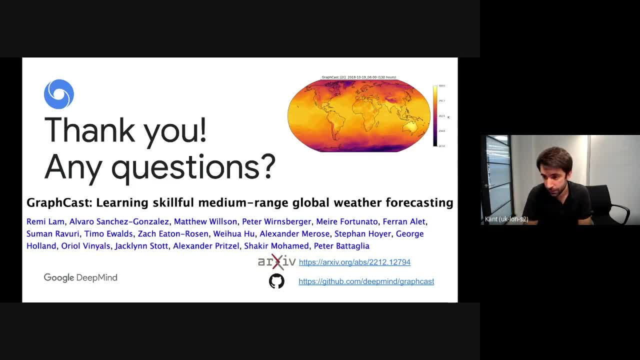 big claim yet because we have no uh published there. so this is interesting. so typically what they do in weather folks, they have an ensemble common filter. have these, you know, 60 miles running. uh, some of them are wrong. pillum kind of push some of the existing population to be to take up the variance of the weather and so on. is that your? 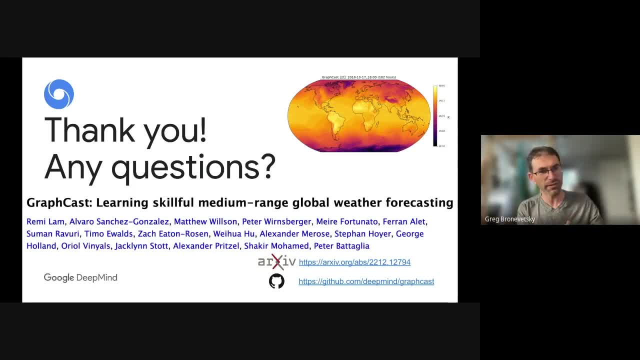 approach, like it's all becoming a filter kind of thing, or the neural nets give you a different way of getting those distributions. oh yeah, in our case there are literally 50 separate predictions if we make them. uh, there's a different question on the data simulation, right? so if you wanted to say, 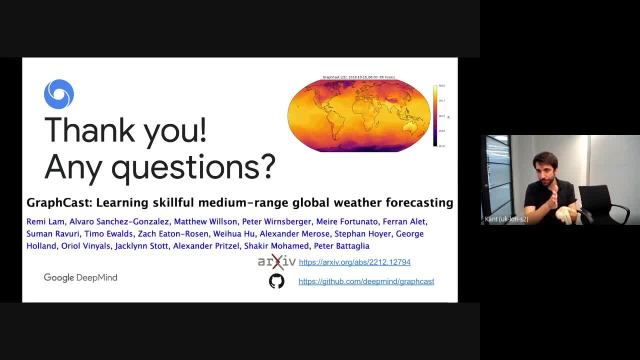 what's the weather state. you would need some form of filtering to eventually come up to the present, an estimate of the present state. we are relying, as i was saying, kind of one of the at the very beginning of the slide. it's not a pure end-to-end ml approach, because the assimilation, uh, the 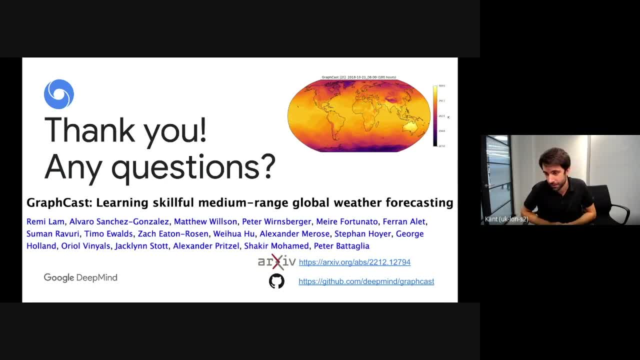 initial state, the input state from which we start, is still nwp based. so i want to make be very clear about this. uh, we're not a pure ml approach and so they are probably running some of the things that you're you're talking about, but but we know we don't on our front is literally